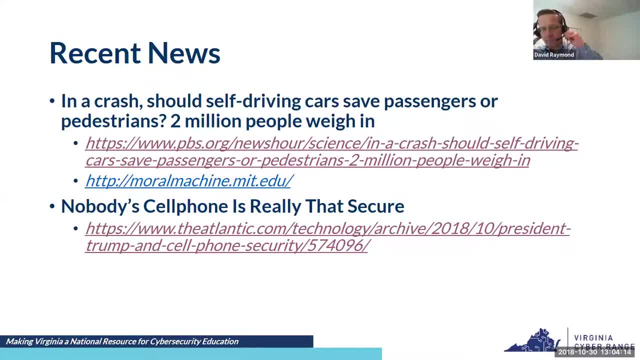 is off of pbsorg And it's so. in a crash, should self-driving cars save passengers or pedestrians? Two million people weigh in, And so this is a story about a study that's been ongoing at MIT for a couple of years, where they have this website, and I'm going to pull up the website, So 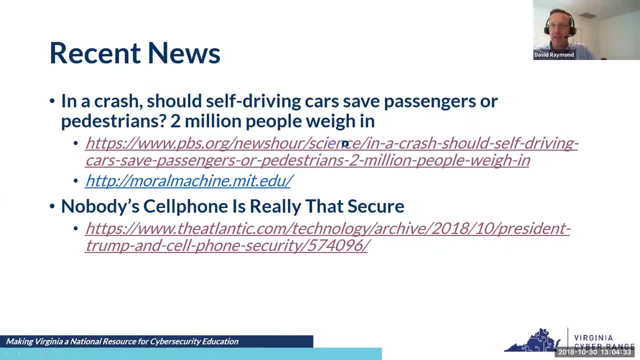 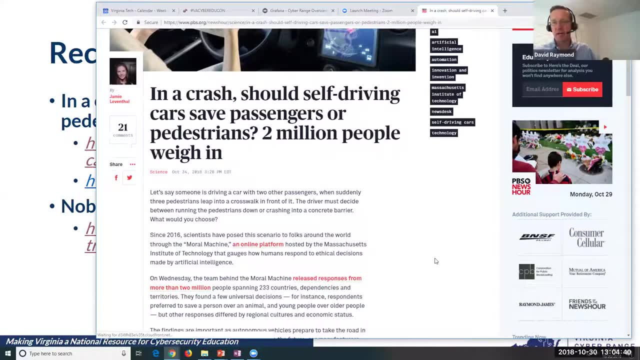 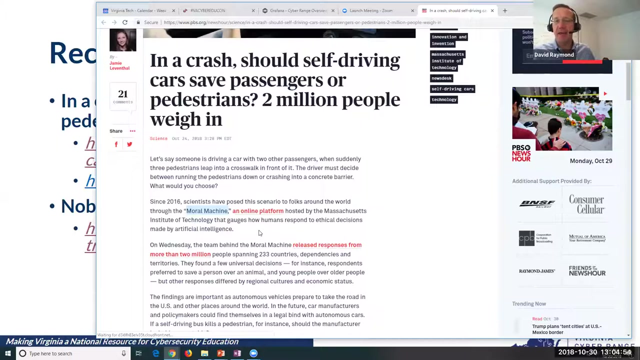 the news story is the first link And if you pull up this link, it's it. you get a bunch of ads, of course, but it talks about since 2016,. MIT has had this moral machine- excuse me, platform running And and it's a- it's a little game that you play and 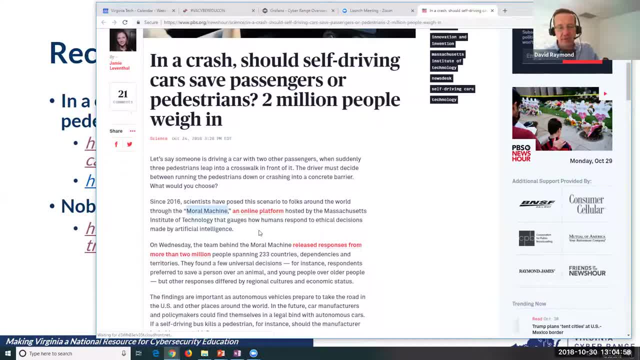 you basically- and again I'm going to show it to you- but but you decide what the self-driving car should do in different scenarios, you know, should it run over the cat, or run over the person, or should it drive into the wall and save the? 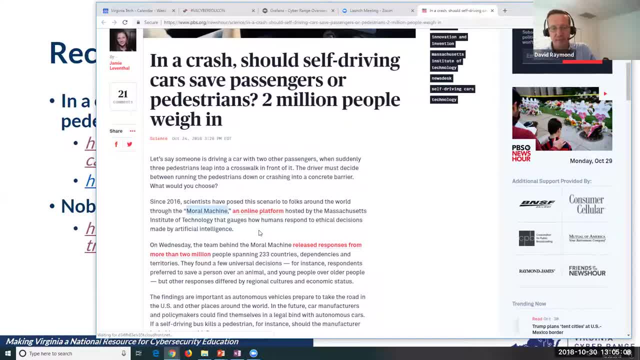 the you know homeless person in the in the crosswalk It's, you know, it's these kinds of sort of you know manufactured ethical dilemmas. But but this is really- I mean, these are really things that, as this technology of self-driving cars progresses, there's going to have to be. 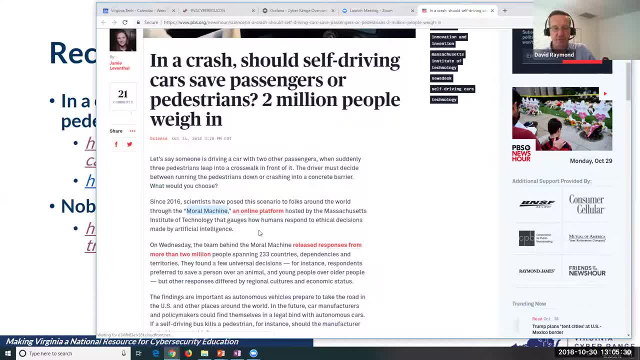 somebody who programs the car to take certain actions in certain situations. And so you know. the question is: when, when something bad happens, who's at fault? Is it the, the occupant of the car? Is it the guy who programmed? 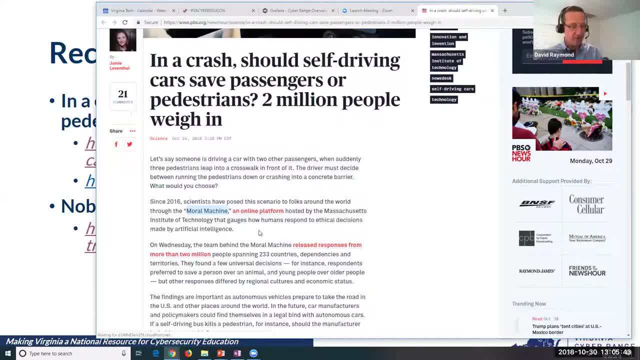 the car? Is it the car? Because there's AI that the car is using to decide what to do. You know so? so that's that's. those are sort of ethical questions that I think are are useful to to get. 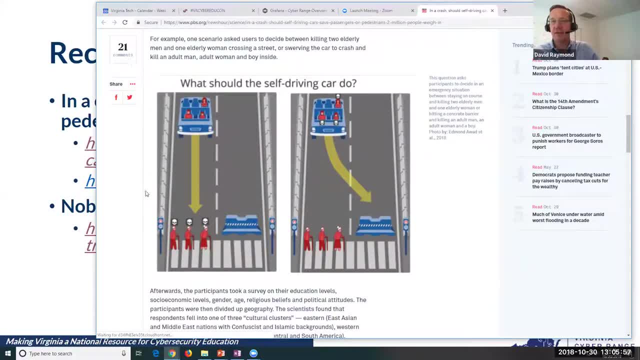 into a discussion with with your students. And so here's a here's kind of a typical scenario. You know, what should the self-driving car do? And so here's a self-driving car, It has three, three people in it, And there's a crosswalk with three elderly people crossing the road. 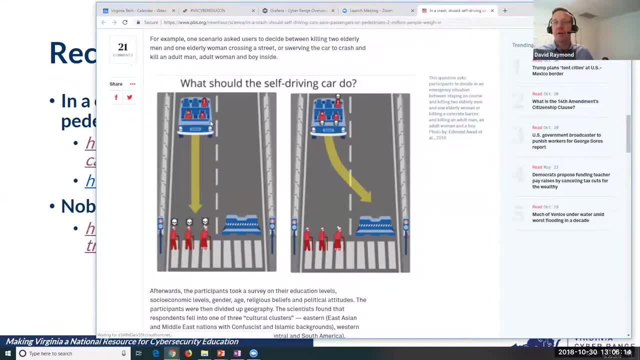 And so the question is: the car is in a, you know there's a. it's at a point where it can't stop in time, And so the question is: or if the brakes failed, or whatever? the question is: what should the self-driving car do? Should it run over the three elderly? elderly people. 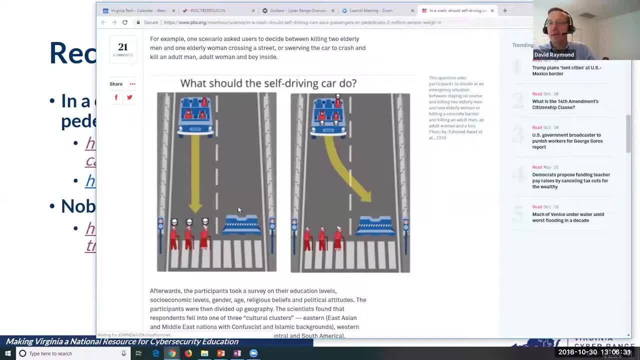 in the crosswalk, Or should it run in intentionally, run into the barrier and kill the three people in the car? And and again, you know it's sort of it's sort of manufactured little dilemma, But but still. 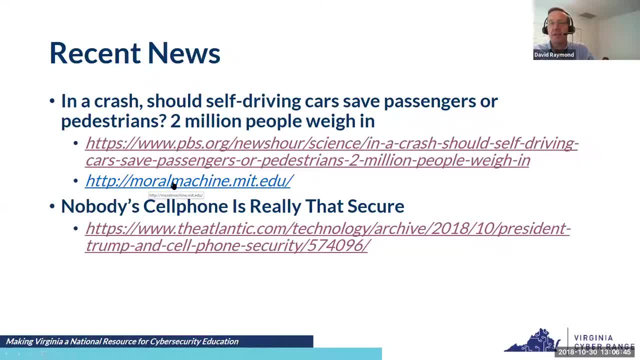 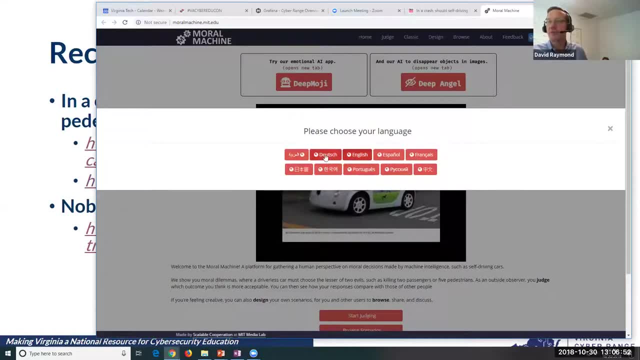 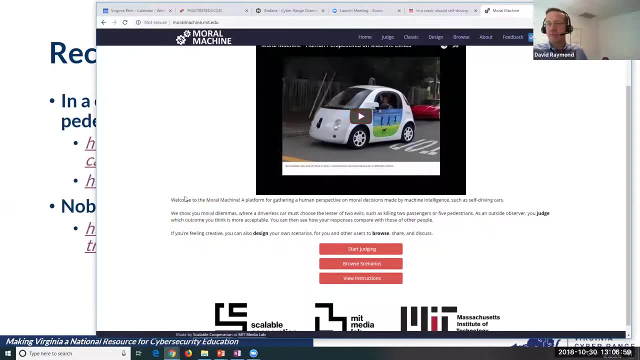 I think sort of interesting to consider. So if you go, so I have the website here to the Moral Machine, http//moralmachinemiteu. And so when you first go here you, you choose your language and then you know there's a little bit, a little movie you're gonna. 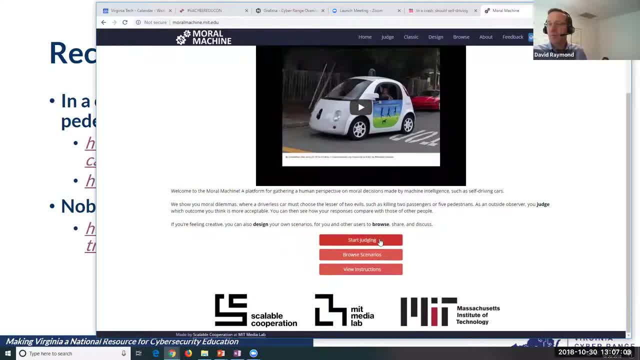 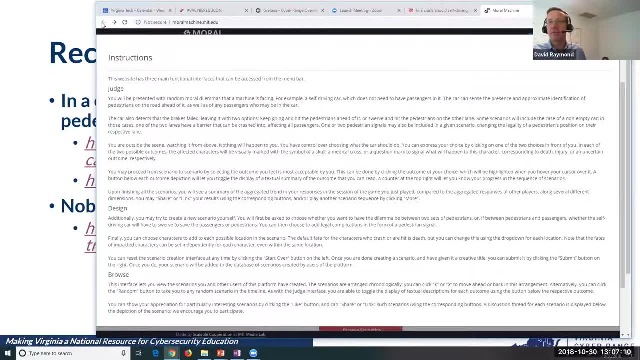 watch about self-driving cars And then you can start. you know you can. you can start judging right. So there's some instructions you can review and you can actually create your own scenarios if you want. but I'm going to- um, I'm going to- just how do I get rid? 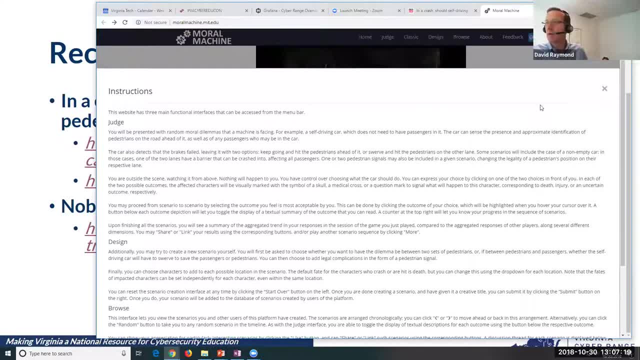 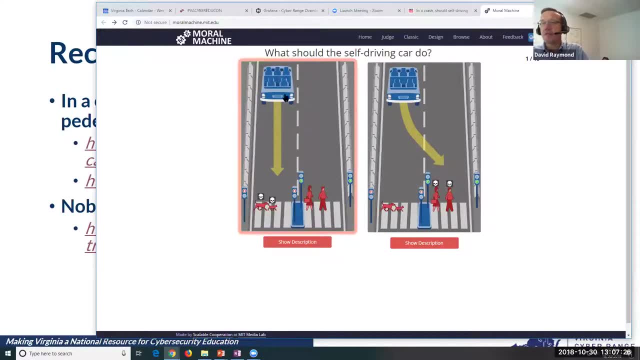 of this darn thing. I'm going to start judging just to show you this. And so here's a scenario: Self-driving car, in this case, is no occupants in the car, or maybe the occupants don't matter. You know, whoever's in the car would, would survive either way. 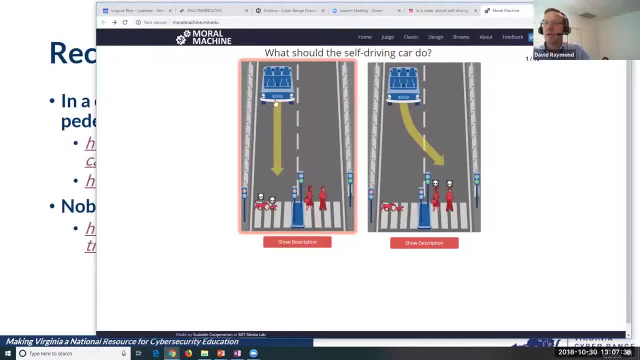 And so the choice is: should the car go straight and run over the cat and the dog, or should the car- oh, and the cat and the dog are crossing against the red light here, if you notice- Or should the self-driving car veer into the pedestrians in the crosswalk that are crossing on a green light? 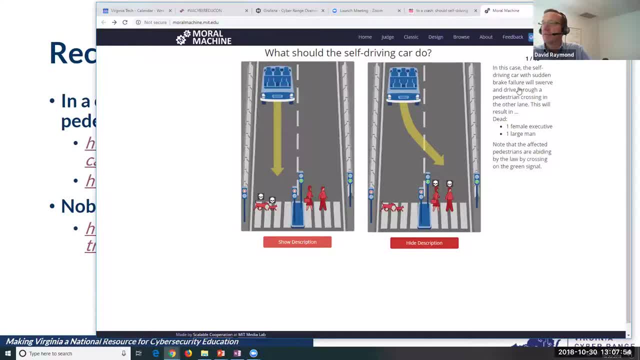 And so you can get a description. In this case, self-driving car with sudden brake failure will swerve and drive through a pedestrian crossing In the other lane. this was in a dead female executive, one dead large man, And note that the affected pedestrians are abiding by the law and crossing on the green signal. 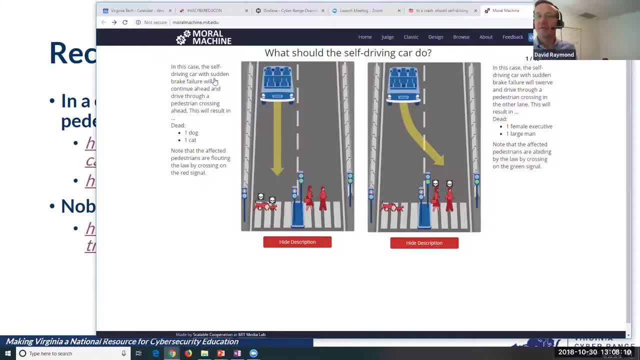 And then over on the left side, you can get a description of this one too: very similar Brake failure car is going to drive through the intersection, kill a cat and a dog, And note that the affected pedestrians- in this case not really pedestrians, but pets- are flouting the law by crossing on the red signal. 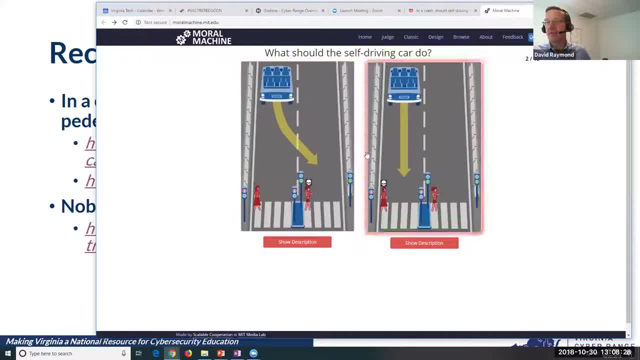 Right. So let's say the car should do that, And then it goes on and gives you different scenarios, right? So again, should the car veer? Should the car veer into the? what is it jogger who's crossing on a green light? 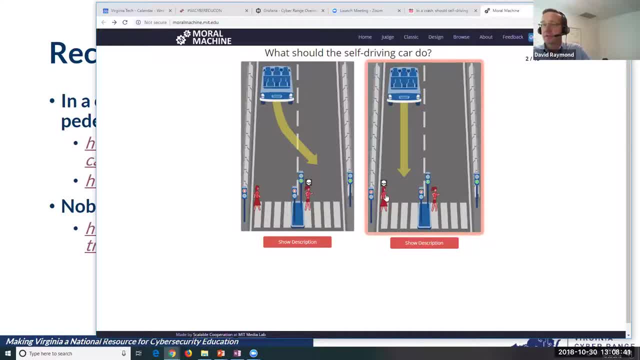 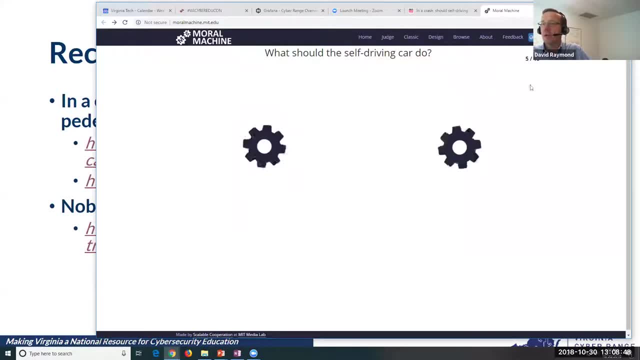 Or should the car go straight and run over the person who is crossing against the signal And you go through? you know multiple of these scenarios. You know you sort of choose what to do And it gives you 13 of them. 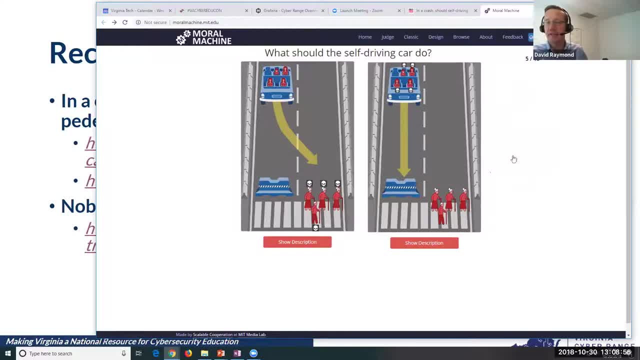 And then at the end it gives you a little. it doesn't you know, it doesn't score. you tell you if you're moral or not, But what it does is it says, It says that you tend to place more value in and it'll you know, sort of give you your statistics right. 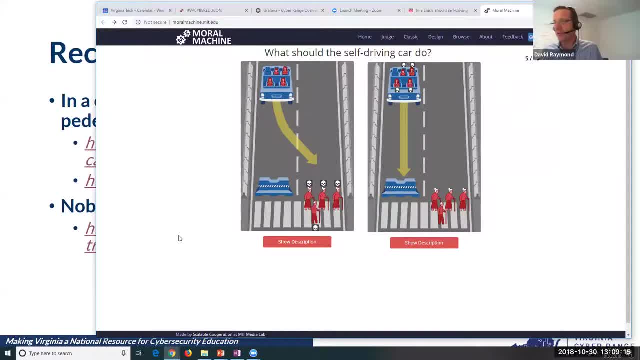 So you place more value in people than you do in pets, Or you place more value in- you know- young people than you do in old people. So interesting exercise, I think, to think about. you know the AI, or you know some decision making that self-driving cars are going to have to do in the future. 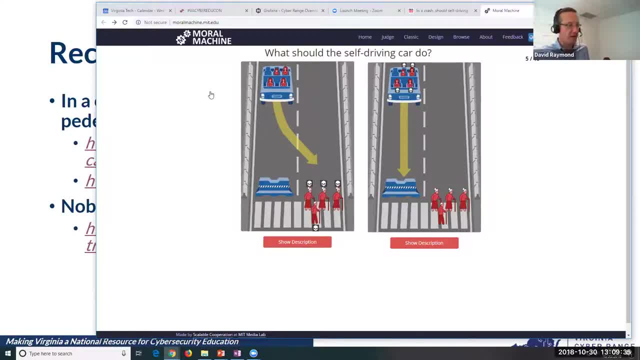 And you know. thus, As far as the discussion of self-driving cars has really been about, are they safe enough? you know so. so are you know. we've heard stories of self-driving cars who have, you know, hit people. 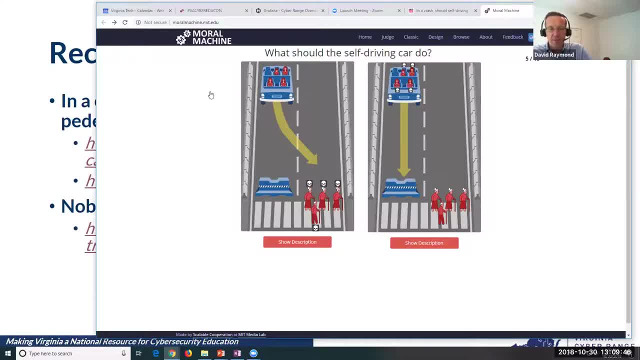 You know there's been, there's been at least one instance of somebody dying because somebody who's not in a self-driving car, somebody who's who is, you know, on the side of the road, who died because a self-driving car, you know, ran into her. 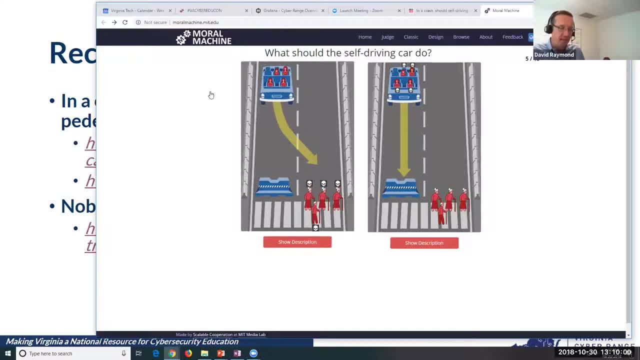 And the person who was behind the wheel, who was supposed to be paying attention, apparently wasn't paying attention, So it didn't wasn't able to hit the brake and cause the car to to stop in time, And you know. but those are straightforward scenarios where the car obviously should avoid the person in the road. when there's, when you know, the other option is, you know, kill somebody. you know it's basically binary: kill somebody or not. 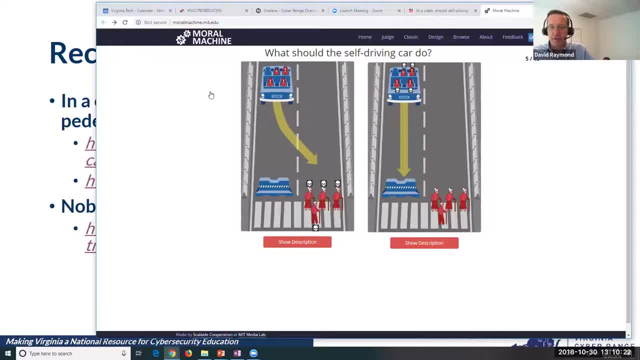 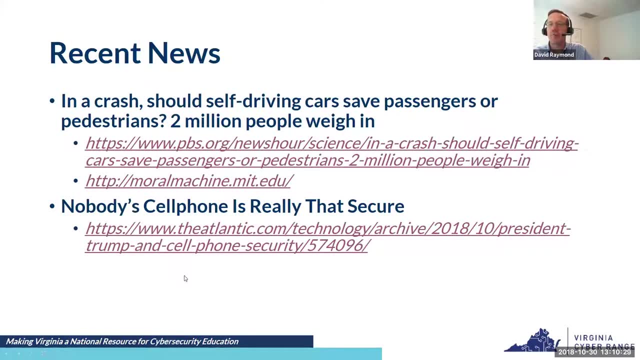 But you know, when you get into these scenarios where you know there's no clear, right answer, it gets a little bit more interesting. Okay, So so that's the first news story. Second news story: Um, nobody's cell phone is really that secure. 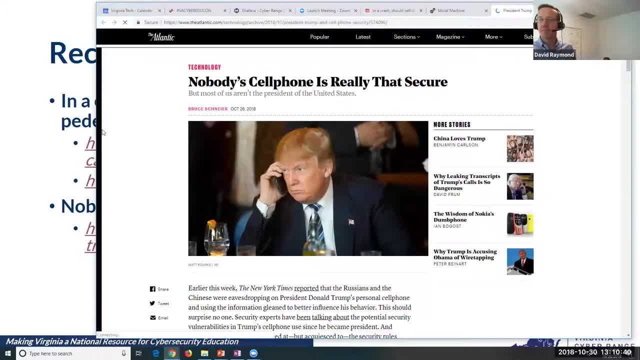 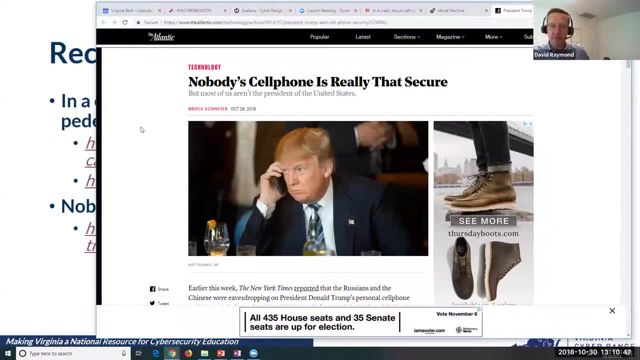 And this is uh um an article in the Atlantic, and it's by Bruce Schneier, who's um. if you're not familiar with Bruce Schneier, he's a security professional- um written several books on the topic. 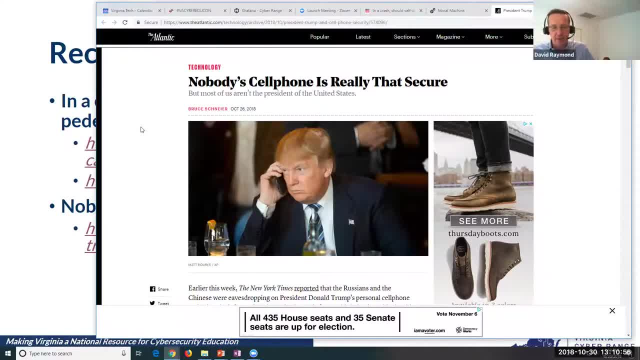 He's. he's considered probably one of one of the one of the leading experts in um information security, you know sort of a visionary. He's written books, both on the technical side. so he's written Applied Cryptography, which is a book about cryptographic systems and how to implement those cryptographic systems in different programming languages. 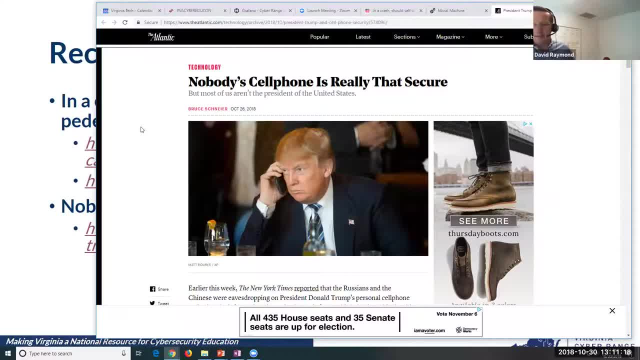 And then he also writes books that have a spin, that's less technical but more sort of ethical issues or privacy issues or those kinds of things. Anyway, so he writes – he has a really good blog and he writes articles and he writes books and he works for, I want to say, IBM. 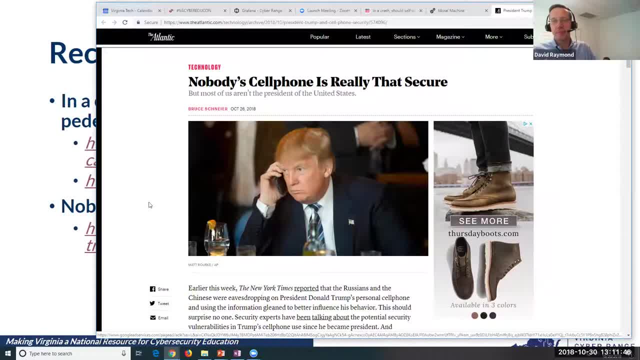 But he writes – so this story is related to President Trump, who apparently uses a – you know he uses a cell phone and that's – you know. so President Obama did the same thing, right, He had a cell phone that he used, and he did, you know, a smartphone that he would make phone calls on. 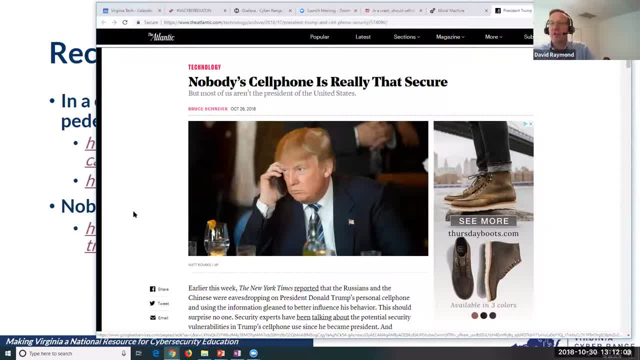 And so in this article, Bruce Schneier talks about the insecurity of cell phones. So nobody's cell phone is really that secure, but most of us aren't- the president of the United States, right? So he describes sort of a list of potential vulnerabilities and you know, they're things that most of us would never really have to worry about. 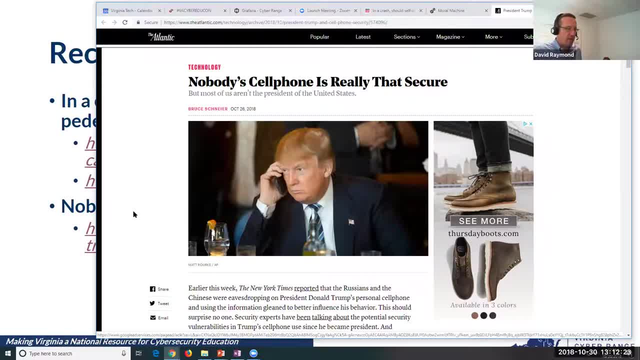 You know we don't – generally we don't have to worry about somebody intercepting our cell phone calls and then doing a man-in-the-mill attack. We can pass that call on to a cell tower, for example, And that's not going to be done at scale to private individuals that we know of. 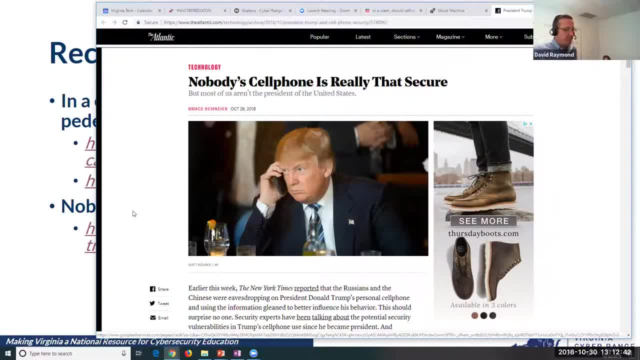 But certainly if you're targeted for a specific purpose, that technology is available and it can be used, and intelligence agencies do this routinely, And so you know. so who should be concerned about this kind of stuff and exactly what you'd think. 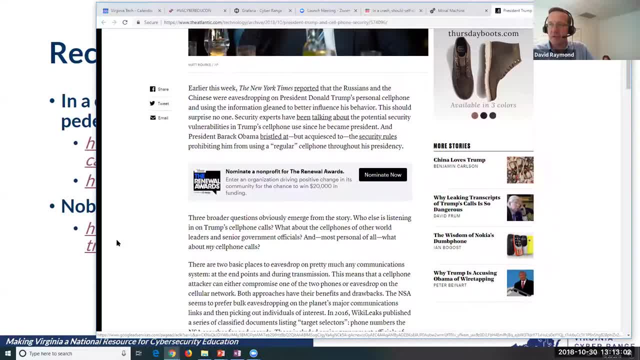 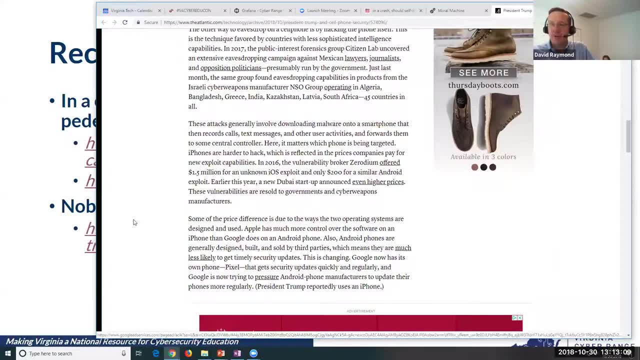 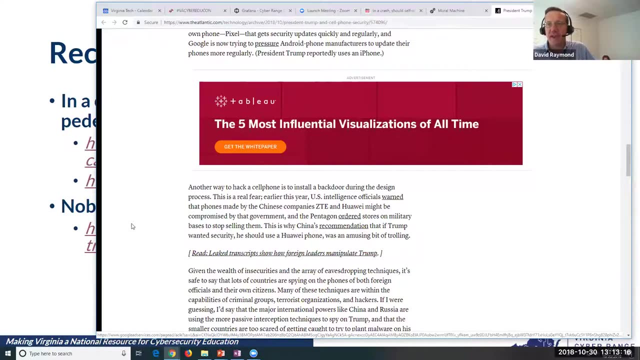 People like the president, Or you know senior-ranking government officials or you know those kind of people. But this is a good article, largely because it – because Bruce Schneier talks about the different vulnerabilities that exist in – both in telephone handsets right. 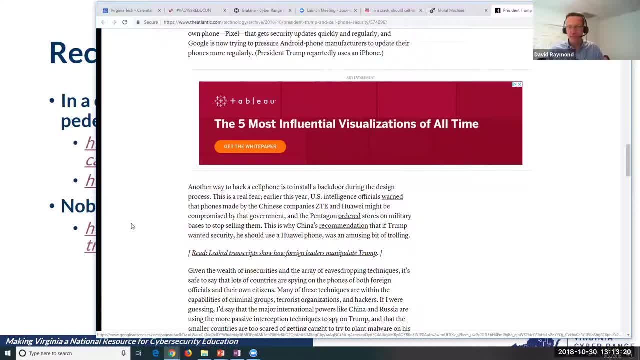 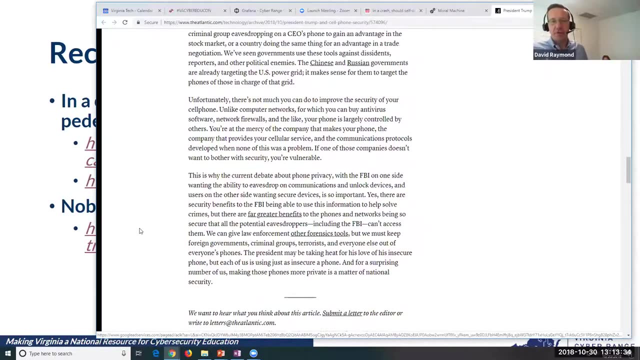 So you have Android handsets, You have two sort of basic classifications. You have Android handsets and then you have iPhones And you know there are different levels of security for different reasons. I think the – I think the sort of understood case of handset security is that iPhones are much more secure. 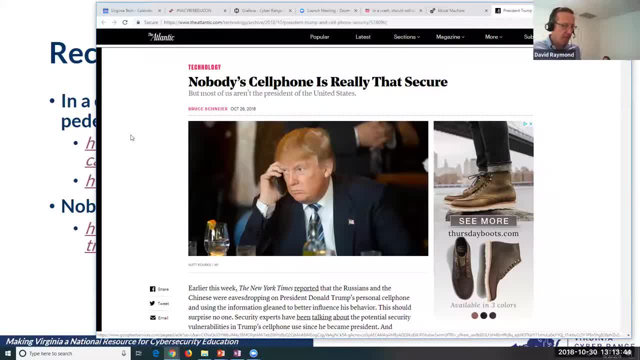 And that's not necessarily because Apple is particularly good at securing their software, but Apple controls the platform and the software, And when you control the platform and the software you can – you know you have a very limited number of devices that the software has to work with. 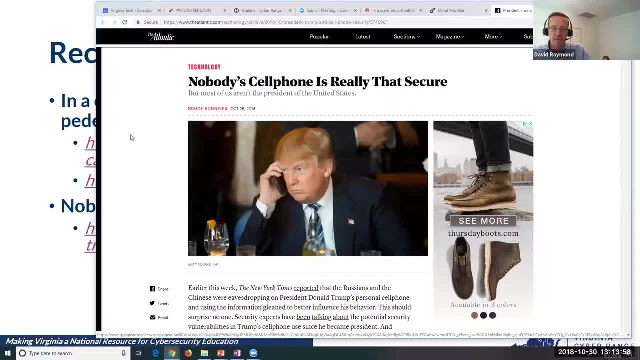 And you can very tightly control what the software And you can very tightly control what the software can do with the platform, which is the phone itself. right, But with Androids, there are thousands of different Android variants, And each Android variant essentially runs its own version of the Android operating system. 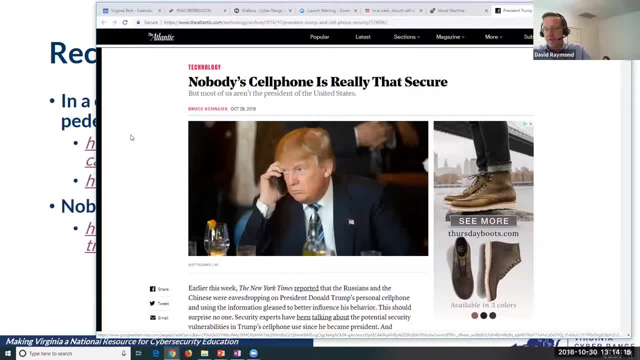 And they're all slightly different and tweaked by the cell carriers and tweaked by the manufacturers of the handsets, And so you have thousands of different versions of Android out there And most handsets – the software on most Android handsets is – Yeah. 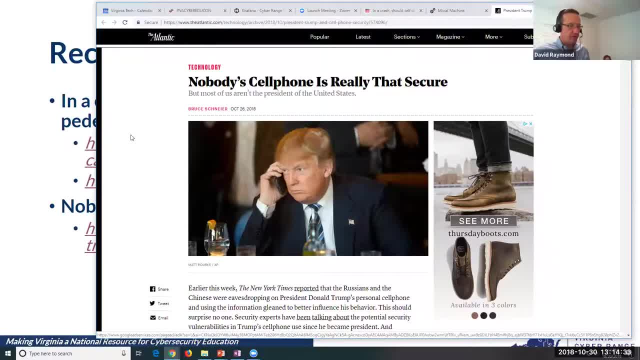 Is only maintained for about a year. So now there are attempts to put laws in place that require that mobile device operating systems are maintained for at least two years, But in most Android handsets that's not the case. They're maintained for about a year. 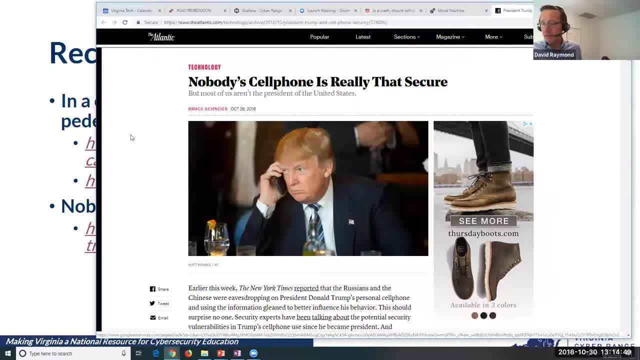 And then after that, if there are new vulnerabilities, you're not going to get a patch With iPhones. you know they're only supporting a handful of different platforms, the different existing versions of the iPhone handset, And so you know they keep that software up to – you know I have a three-year-old iPhone and I just got the latest iPhone software update, you know, a couple of weeks ago. 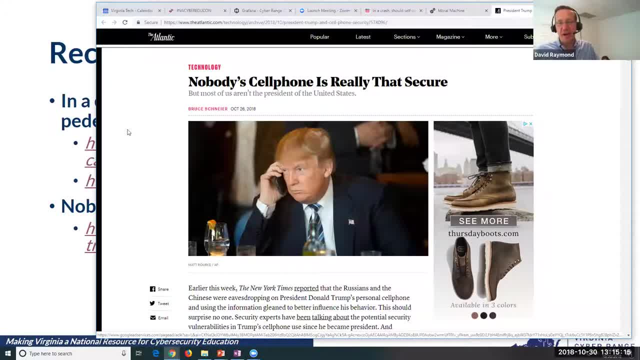 So it's just easier for Apple to keep it secure and to keep the software updated. But it's not only the handsets and the software that have security issues. There's also issues related to the cellular system itself. right, So I mentioned you could potentially eavesdrop. 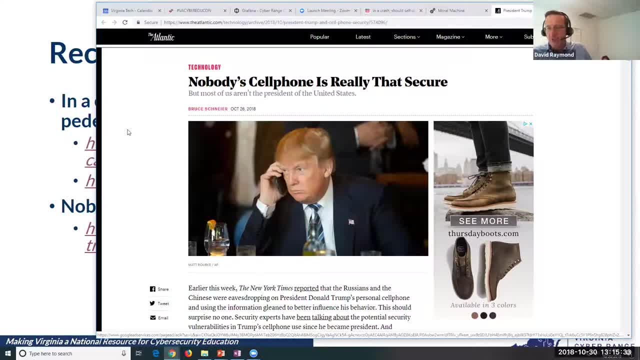 On a cellular telephone or conduct a man-in-the-middle attack on a cellular telephone call, because it's just a radio signal. Of course it's encrypted. But if you do the right kind of man-in-the-middle attack, then there's potential to do this thing where you set up an encrypted connection between the handset and the man-in-the-middle. 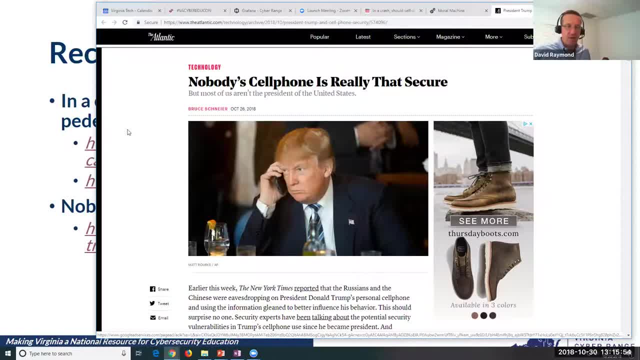 And then you set up another encrypted connection between the man-in-the-middle and the cell tower, so that the handset and the cell tower don't realize that there's somebody in the middle who's actually listening to the conversation Or eavesdropping on the network traffic. 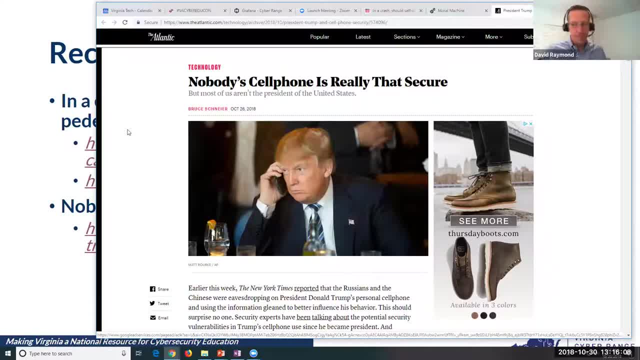 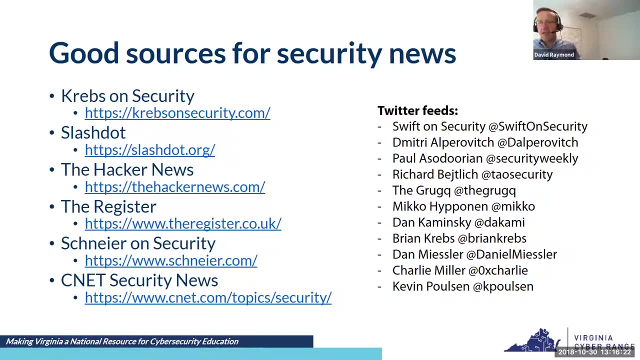 And again, you know, nation states certainly are in a position to do that kind of thing. So good article. I think Okay, So that's enough news. So a couple of weeks ago, three weeks ago maybe, I thought it might be helpful for folks to throw up some sources of security news. 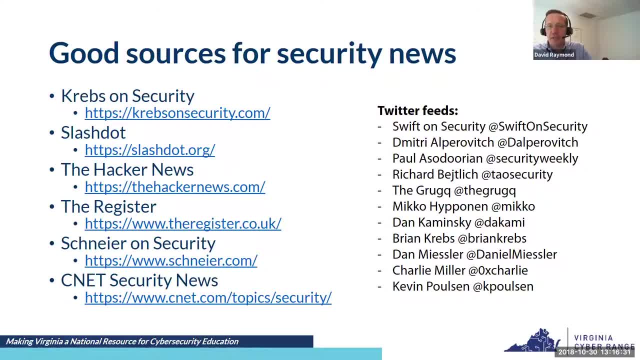 This is the same slide I threw up three weeks ago. I'm just going to throw it up again quickly because if you haven't seen it before, you might take a screenshot and then use this later. So it lists some good security news sources on the left and then Twitter feeds on the right. 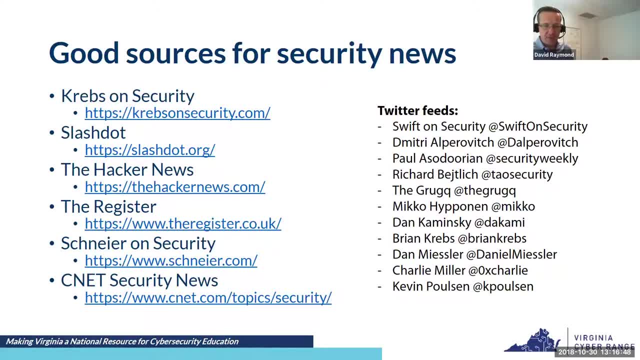 InfoSec people are Twitter people. So you know, I think there are certain groups of people who are active on Twitter And you know, I know it's like a thing for celebrities and athletes to do Twitter. It just turns out. 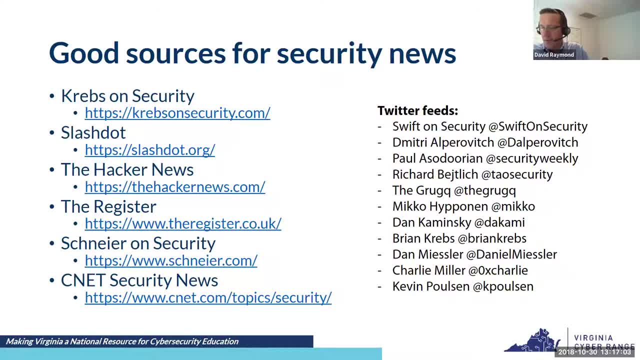 It turns out that InfoSec people are also Twitter people, So there's lots of good Twitter feeds within the InfoSec community And, if you do it right, you can filter your stuff so you only get the InfoSec stuff and not all the other useless garbage. 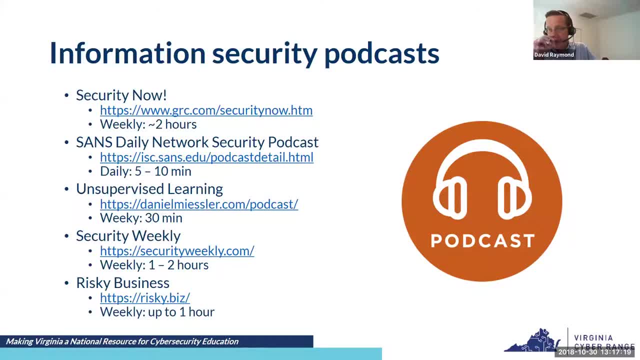 So, anyway, news sources and Twitter feeds, But I added to that some InfoSec podcasts, So I'm a bit of a podcast guy. I spend a lot of time on the road driving around the state of Virginia, And so when I'm driving around I listen to podcasts. 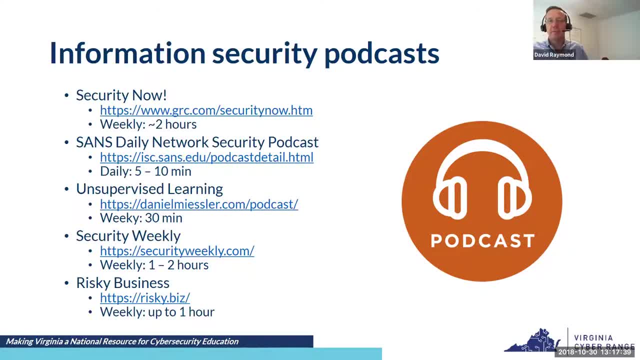 And so these are some some that I think are pretty good. Security Now listed at the top there, That's a weekly podcast And it can be up to two hours long, but it's recent security news and then some additional context to make that news more useful. I guess, is how I describe it. 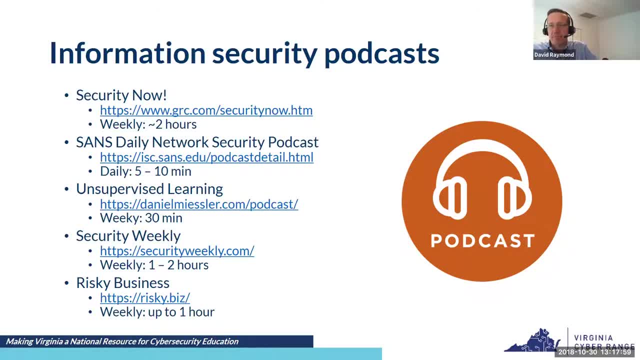 But it's pretty good, Very, very well regarded InfoSec podcast. Second one: SANS daily network security podcast. This is a daily podcast. It's very brief, but it's- and it's really, I guess, mostly intended for InfoSec professionals. 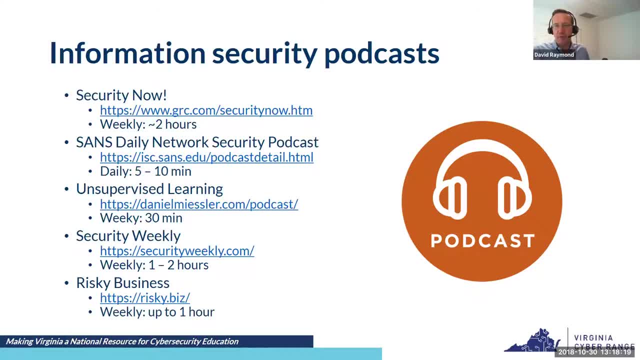 So maybe educators wouldn't listen to it so much. I don't really listen, you know. Once in a while I pick it up And if I know of a recent exploit or recent interesting vulnerability that I don't know a lot about, then I'll jump on the SANS daily network security podcast. 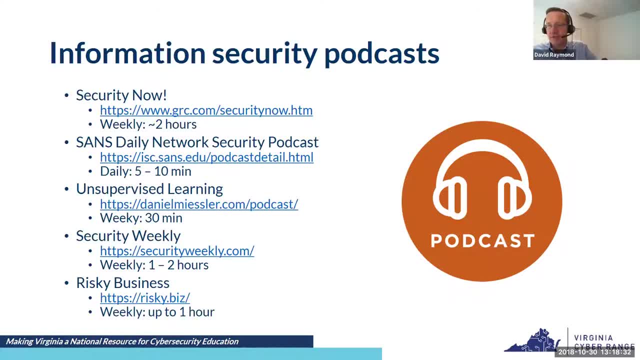 I pick it up and if I know of a recent exploit or recent interesting vulnerability that I don't know a lot about, then I'll jump on the SANS daily network security podcast, daily network security podcast And- and you know, they usually do a podcast on those things- 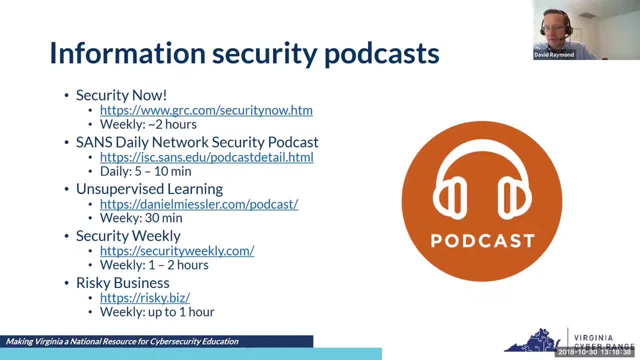 like the next day or two days later, and you can get sort of the the, the meat and potatoes of those interesting new exploits very quickly. So again, it's only five or 10 minutes long. The next one on the list, they're unsupervised learning, So that's Daniel Meisler, who's a 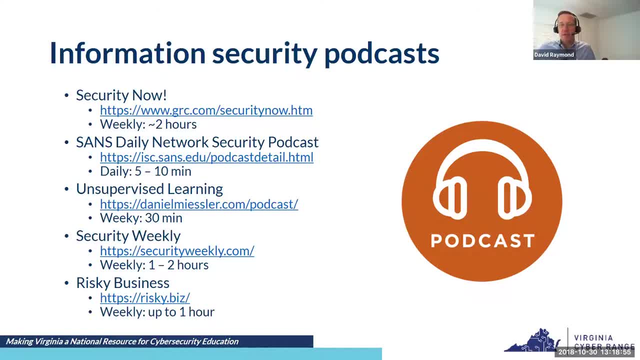 another pretty well-known InfoSec professional. He does this weekly podcast and he really distills a lot of. he really distills a lot of recent security news into a you know sort of a 30 minute. So it's not a lot of fluff, It's. it's really just, you know, pretty well distilled. 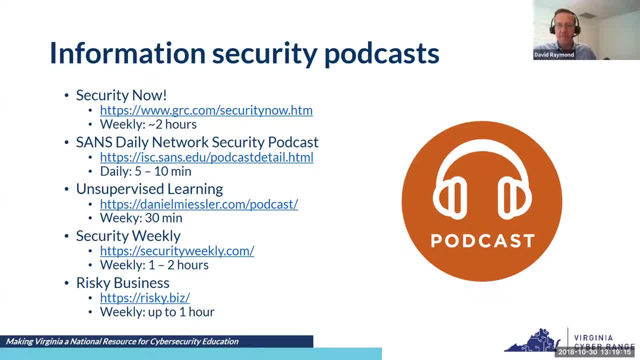 information into a 30 minute podcast every week, Security Weekly, the fourth one on the list there This is: this is a podcast by Paul Asadorian and some other folks, that sort of come and go. He has this group. He has a group of six or eight different people that that you know join in some weeks and not. 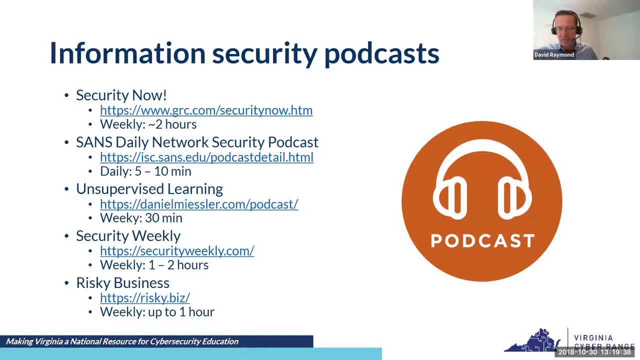 other weeks And- and this is a group that's pretty active on like the, the HackerCon scene, So you know you'll see Paul Asadorian and Joe Pesci and, I'm trying to think, some of the other folks. you know a group of people that that you know. you know I'll see him at Black Hat. 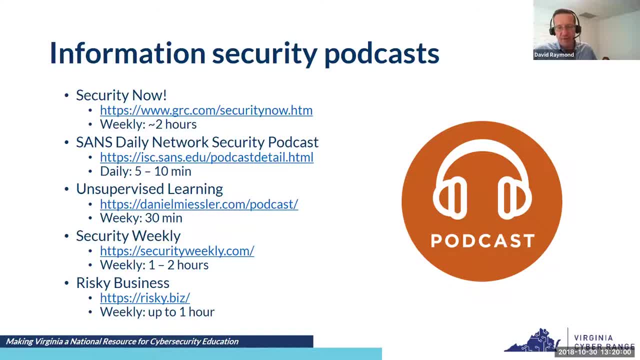 every year They'll be at at DerbyCon And at the different B-Sides events, And yeah, so Jack Daniel is another one of the three or four people who are sort of on this podcast most weeks, And then there's some other people that come and 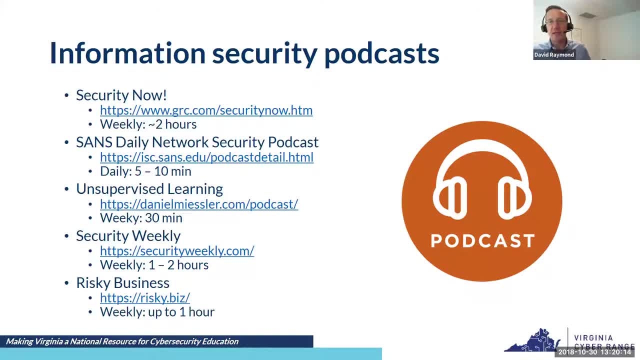 go. But but so this is a. this is one to two hours every week. It can be sort of not safe for work. You know, sometimes they- I mean they- don't use a lot of profanity, but they'll, you know. 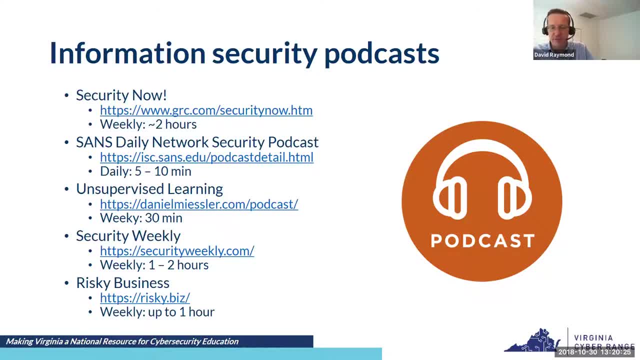 talk about, you know, drinking too much at a conference, or you know things that maybe your high school kids wouldn't you know, maybe you wouldn't want to Expose them to it, But but it's but they have. you know they'll have people come in from. 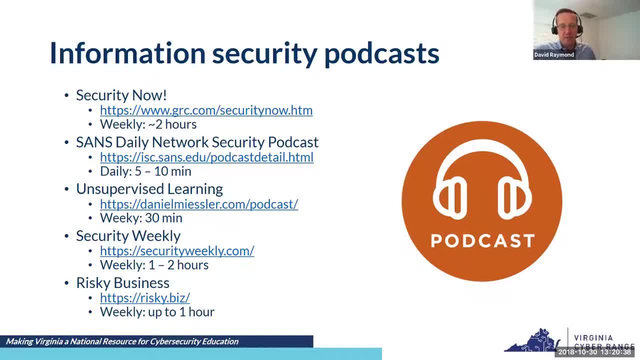 different security vendors and they'll sort of grill them on their, on their security tools And and I mean it's it's pretty good. They usually have a you know in and amongst the the other stuff, they usually have a really good discussion about recent. 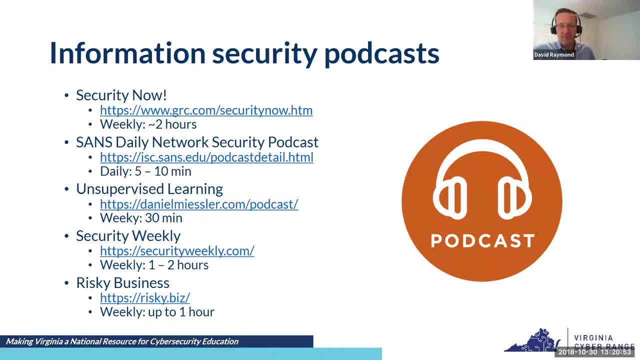 things going on in the InfoSec community. And then the last one risky business is. so that's a one hour weekly. I've I've only listened to it a couple of times, You know I my recollection is that it's is that it's pretty good. You know pretty well. 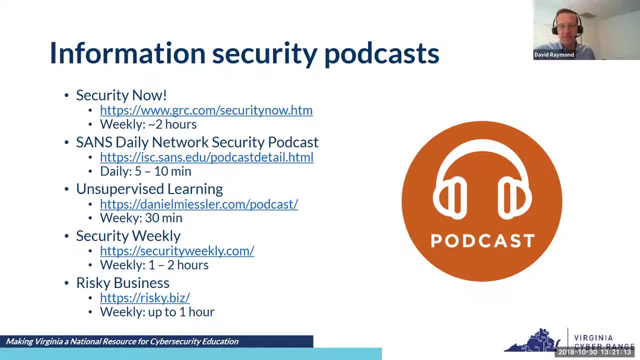 distilled useful information, not a lot of fluff, But I'll I add that to the list as well. I'll say security weekly, the, the fourth one. there is a lot of good content but also a lot of fluff. 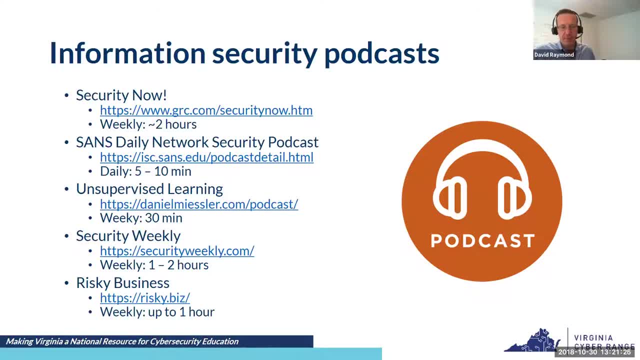 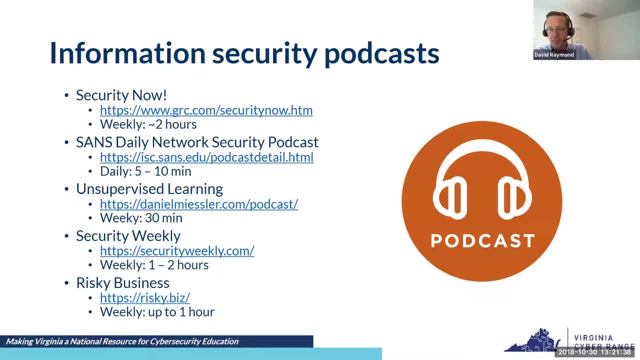 you know, security InfoSec people are podcast people, So this is a good way to- if you spend a lot of time in a car, this is a good way to to kind of stay, or, you know, if you get on the treadmill or or whatever good way to get some InfoSec news where you don't have. 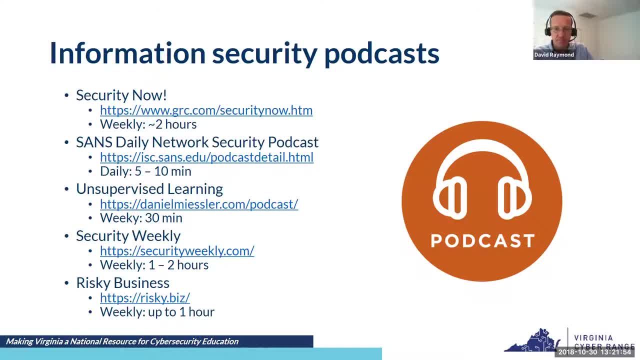 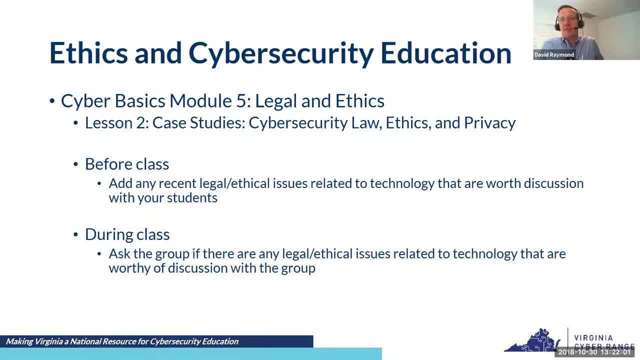 to you know, spend time on a website. Okay, So today is we're going to be talking about ethics and cybersecurity education. So this is directly from the cyber basics course in the course repository, module five, legal and ethics lesson two: case studies: cybersecurity law, ethics and privacy. So I just pulled the slide deck straight out of there And that's what I'm going to use today. 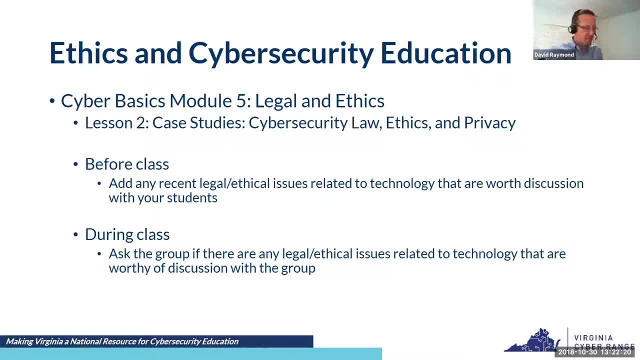 What I would you know once I go through this you'll you'll probably get some ideas on how to use this content in the class. The way I'm going to present it is the way I sort of do it at at. 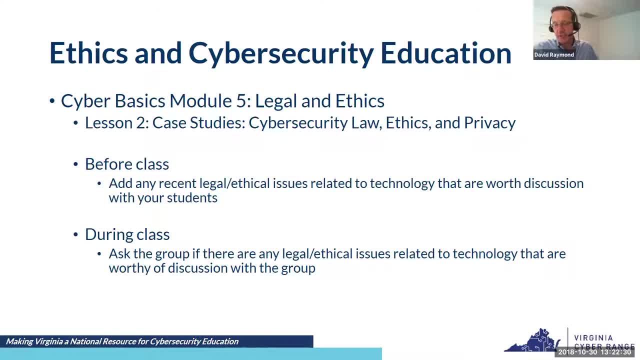 GenCyberCamps With high school teachers, but it's that's kind of the way I would approach it with students. Also, if I was, if I was doing this with a group of students, you know, what I would suggest for for you teachers is to you know, before you use this in class, think about any recent legal or ethical issues. 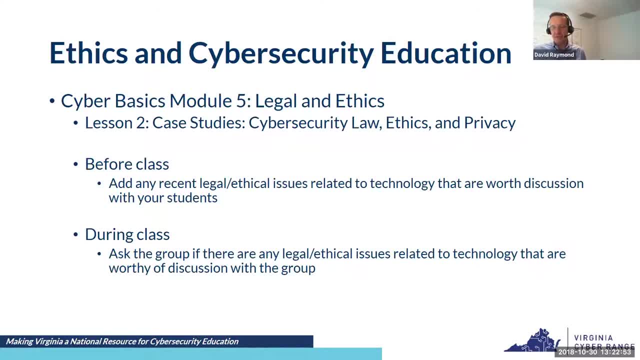 that you might use as case studies. So this is really a series of case studies. And then I would also ask students, you know if you're going to use this, even if, even after you add your own case studies, I would sort of throw it out and say, okay, how would you? 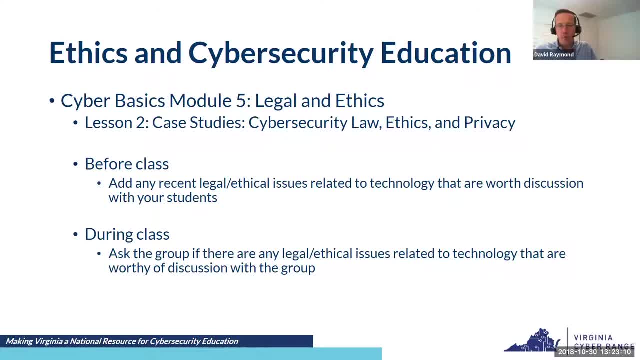 How would you What, what topics might you add to this list, kind of a thing. and And actually I have. I was just having a chat with my daughter yesterday who's in AP computer science fundamentals course in high school in Virginia And she has an assignment where she has to. 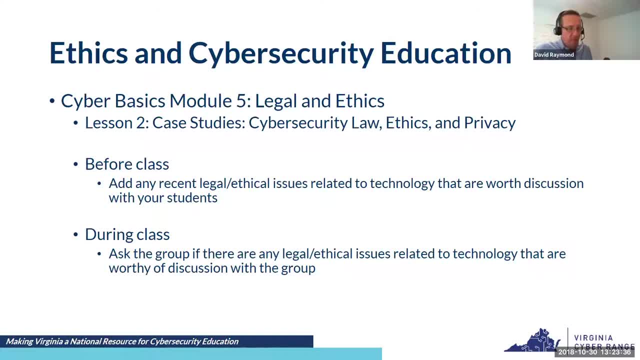 Select a recent advancement in computing and And then sort of talk about pros and cons From all angles, and you know. so that's one way you can approach this kind of an assignment or a discussion. And then I guess the idea is that students will pick different things and then, and then the group will come together and talk about these, these different, 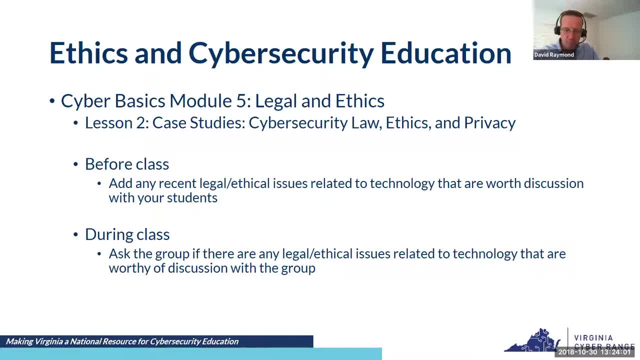 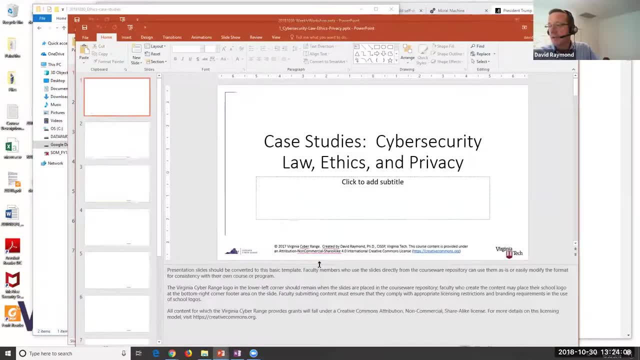 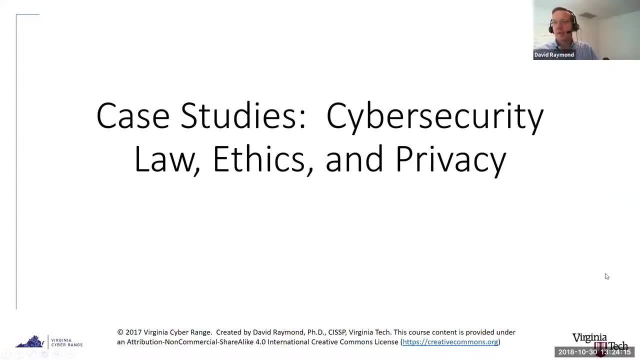 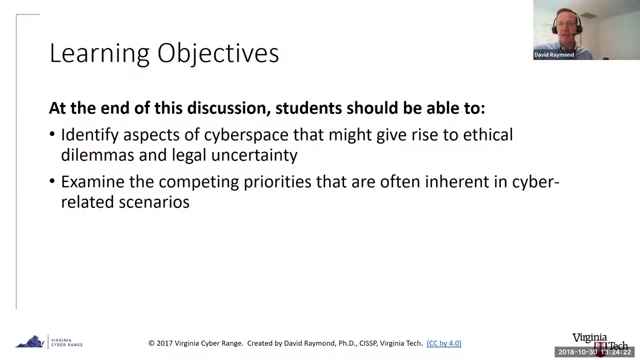 Developments and And the pros and cons. Okay, so You find my other slides. Okay, so it's a 25 minute build up. All right, here we go. Cybersecurity law, ethics and privacy. Couple of learning objectives: students should be able to identify aspects of cyberspace that might give rise to ethical dilemmas and legal uncertainty, and. 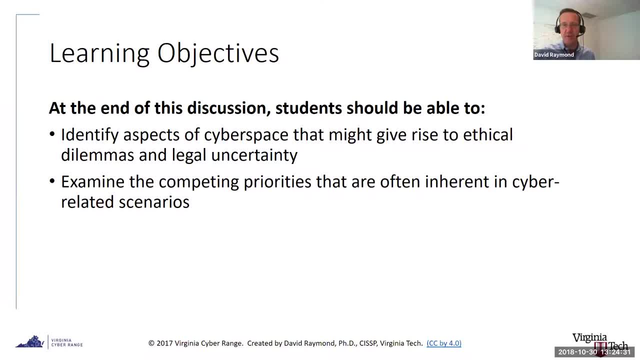 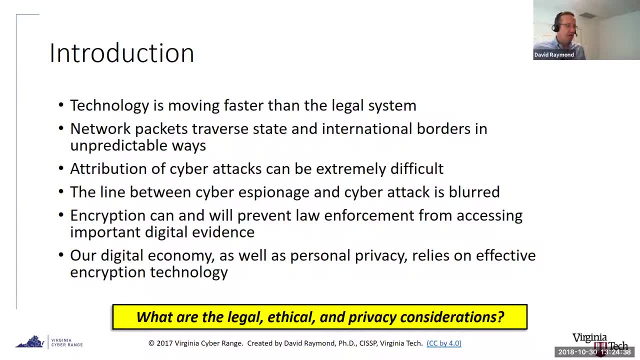 And then examine the competing priorities that are, that are often inherent in cyber related scenarios. So this, so this is So again, series of case studies. but I start with this slide And I think it's helpful to sort of set the context of the case studies. 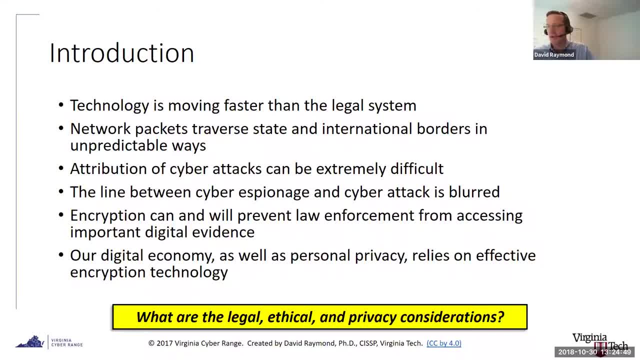 So the first bullet here: technology is moving faster than the legal system, And I think That's always been the case, Right? So you know, anytime there's a new technology that's introduced, It always takes a while for the laws of law to change. 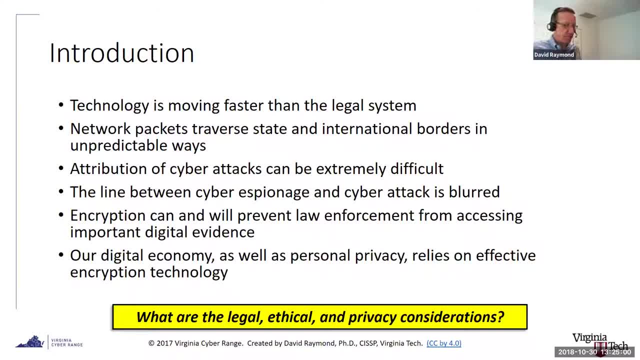 It takes a while for the laws to catch up and you know, historically technology moved at a at a slower pace And so you know you'd have this period where the laws weren't quite catching up, but But you know generally wouldn't take long. laws would catch up and then the technology would go on, you know, relatively unchanged for a long time. And if you think of like traffic laws, right, you know cars started becoming popular in the, you know, early 1900s. 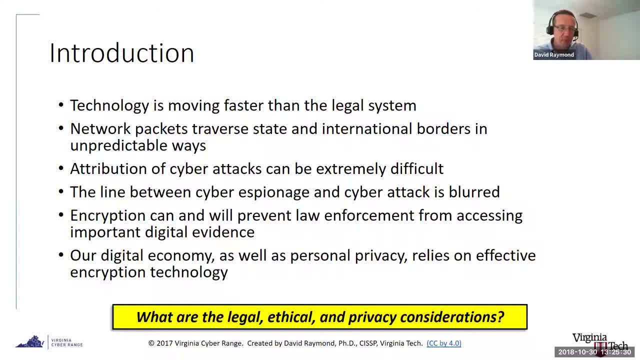 And You know there was concerns about the speed of cars. So there were, in some places are laws that said the car can only, you know, couldn't drive faster than 10 miles an hour, because you can go faster than a trotting horse, or it would be too dangerous. 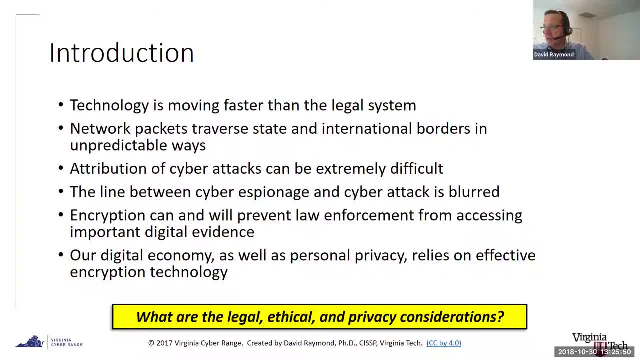 There were laws that said you couldn't drive a car unless you had somebody walking in front of the car to warn people that the cars coming, You know. so you had these, had this new technology, And then you had some some interesting reactions to the new technology. but you know, over the, I think, pretty quickly. 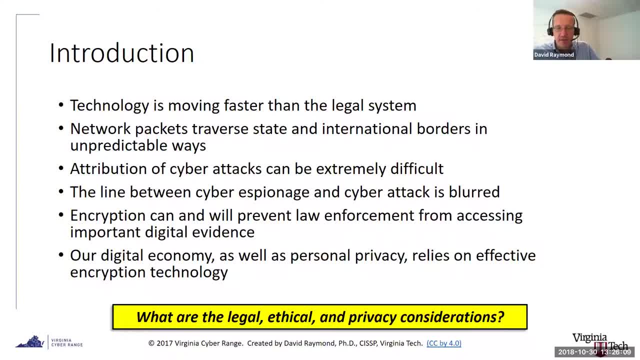 There were some clear traffic laws. you know right of ways on certain types of intersections, different signage that would be used to. you know whatever stop signs, yield signs, etc. You know speed limits and You know and those laws probably solidified, I don't know, maybe in the 30s and 40s. 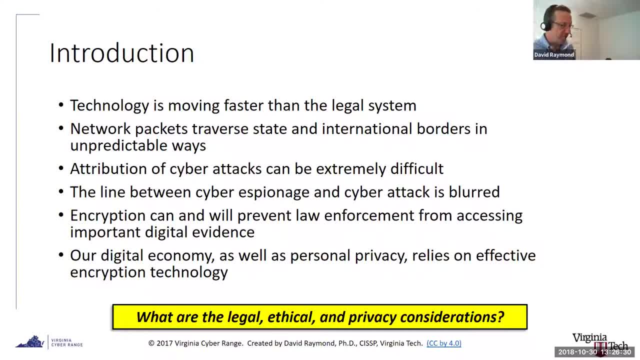 And that's essentially remain. you know, most of that stuff has remained largely unchanged, you know, for the last whatever 70 or 80 years. But with with the advancements in technology, That's just not the case anymore. You know things, things happen too fast and 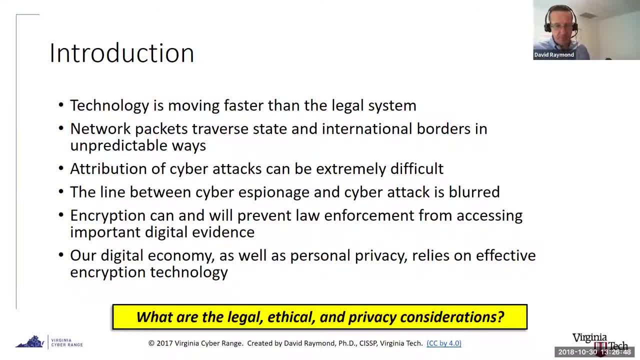 And you know, by the time the laws catch up, You know the technology is sort of moved on and many cases So technology moving fashion, the legal system, Second bullet there, network packets. So you know there's a whole bunch of different ways that we can use the law to reverse state and international borders in unpredictable ways. Okay, so why is that relevant? 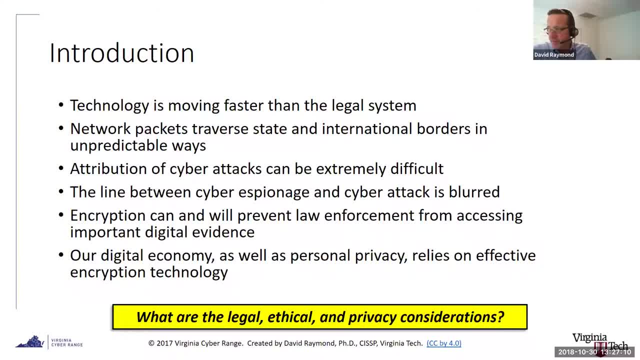 Well, so so students who have taken, You know, high school civics classes, for example, you know they probably understand the difference between State laws and federal laws, Right? so so you know if a, if a crime happens in a certain jurisdiction, then there's a local 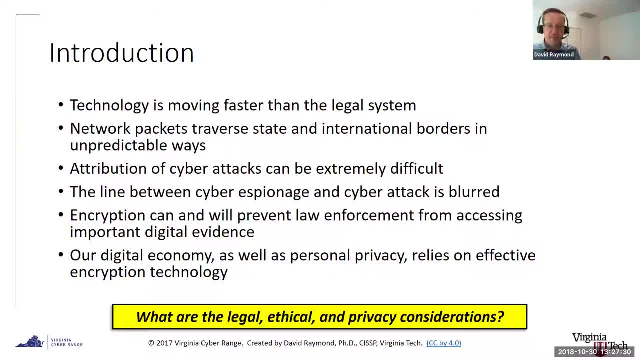 The state is responsible for enforcing the laws in that jurisdiction. But if a crime occurs that crosses state borders, then all bets are off Right. So now the jurisdictional issue is a federal jurisdictional issue, not a state jurisdictional issue. So now you have, you know, you've elevated the generally elevated the severity and you've 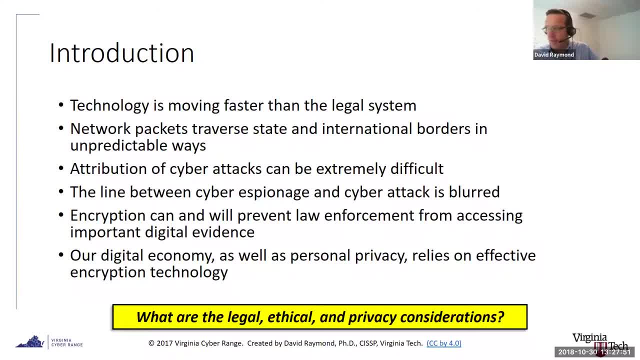 And you've changed who is going to investigate and how, how they're going to be prosecuted and etc. and So that's the same with with international borders as well, And it's more of a, it's actually more of a concern with international borders. 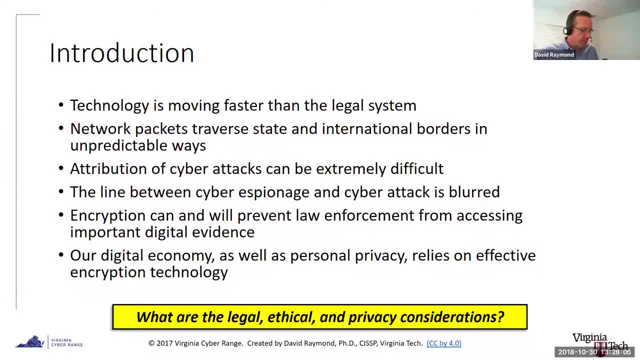 And an example I'll use is, If you recall, in the in the late 80s, the US launched a bombing mission against Libya, against Muammar Qaddafi, and I think it was- I'm pretty sure it was- Qaddafi in Libya late 80s. 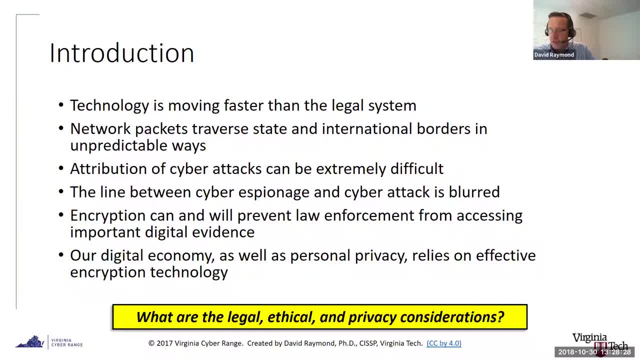 President Reagan, I believe Maybe it was Bush They launched this Attack to, For whatever reason- I don't recall the whole story- but gonna bomb Libya right. and so they were launching aircraft from the UK and they had to fly over several countries to get to Libya and 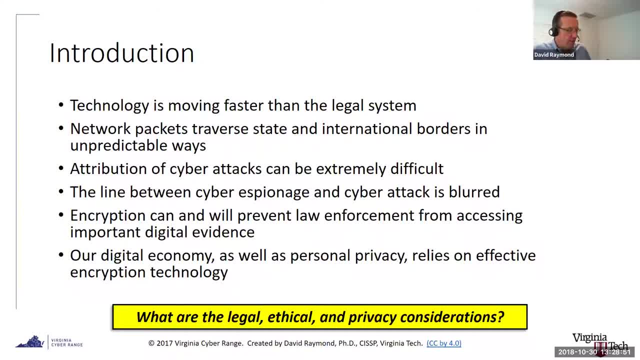 Before they did that, they had to get permission from each one of those from the airspace, from each country through which the aircraft are going to fly, because they were going to conduct a, An offensive military mission against another country. And so the US had to get approval from each country over which these aircraft are going to fly. and the French said: No, you can't do that. You can't fly through our airspace to attack another country. And so the 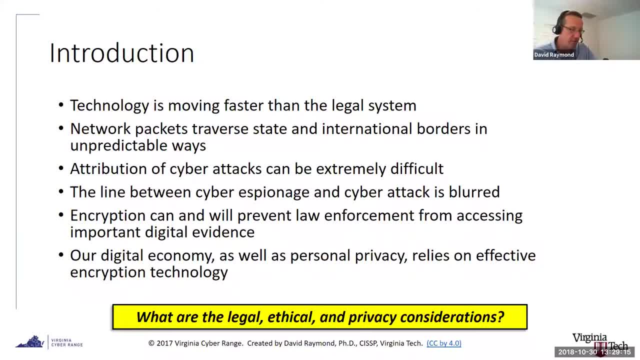 Course the attacks will happen, but they had to fly a different route- you know longer distance- to avoid French airspace. and if they would have flown through France to conduct this thing, then then the French could have. you know, there's international law that says: 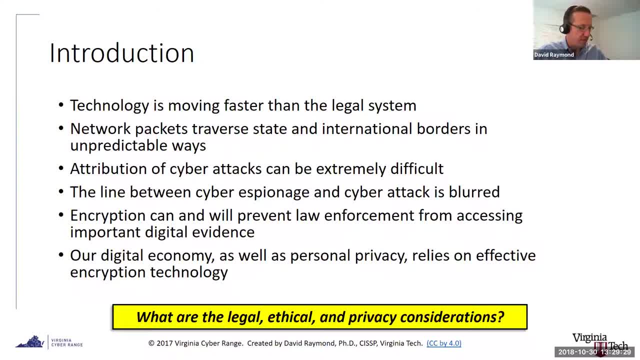 You know you can't do that without the permission of the country involved, and And so, in the case of the airplanes, It was easy for the US to take care of that. fly around France right now. in cyberspace, Things are different. Right, If we're going to conduct a cyber attack against another country. 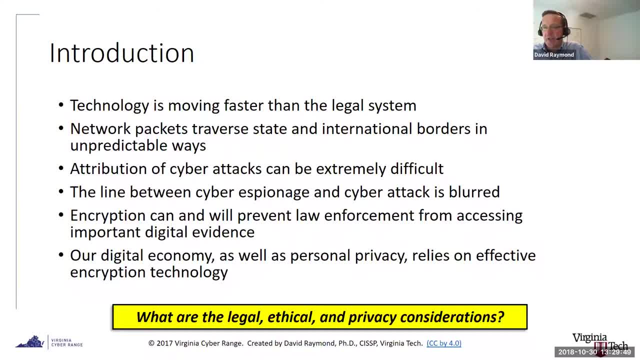 You don't know the route through which those network packets are going to, are going to take to reach their target. you know the internet is designed To route packets On the most efficient route and there's really, there's really no practical way to to specify the route that the packets will take. 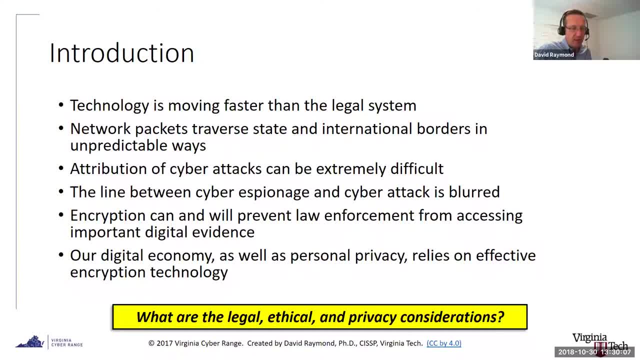 So if I conduct a cyber attack against Libya from the UK and I can't control the countries through which those packets traverse, Am I violating international law by doing that? if the, if other countries say no, you can't attack through us. So I think that's just one example of of. 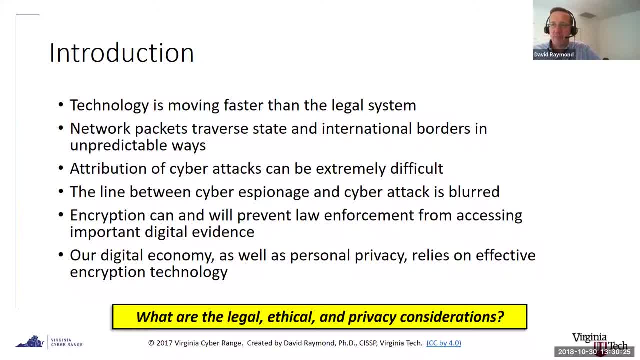 One of the repercussions of the fact that network packets, You know, Traverse borders in unpredictable ways. Another example of that is The fact that You know you don't know where your packets are going to go, So your packets may end up going through a country that is hostile to you, or to you or to your allies. 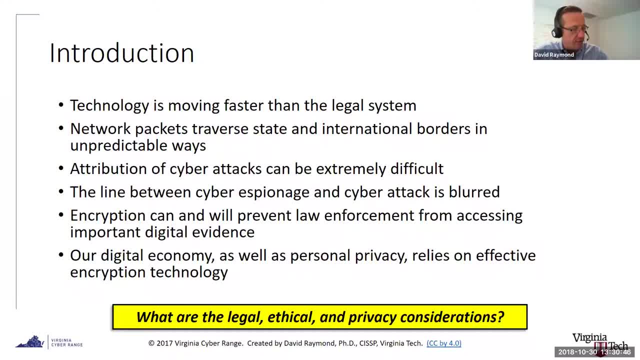 And so if the packets are traveling through that country, then that provides an opportunity for eavesdropping right, so that country could intercept all those packets along the way and then try to decrypt them if they're encrypted, or read the traffic If it's not encrypted. 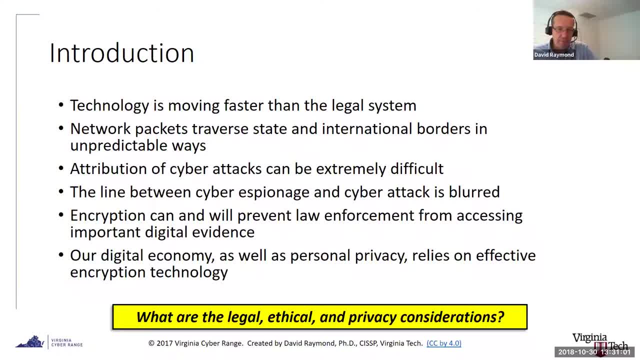 And there are actually instances where There's one specific instance that's pretty well known from, I don't know, seven or eight years ago, where a major portion, something like 25%, of all worldwide network traffic was improperly routed through a specific region in China. 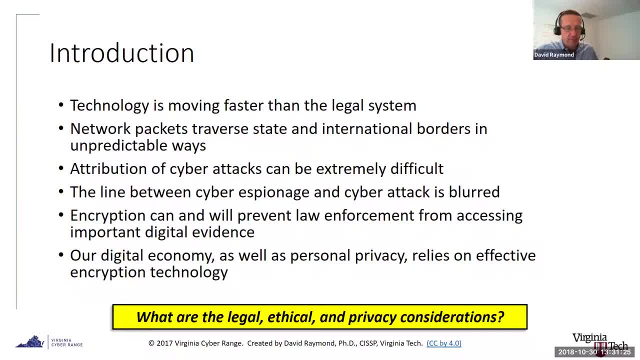 And, and that was based on A Misconfigured routing equipment in China. And so so this thing was this, the fact that this was happening was discovered, and A lot of people pointed fingers at the Chinese and said, Hey, how come you're purposely, you know, routing all this traffic through your infrastructure? and the Chinese said, Oh, you know, it wasn't purposeful, It was a, it was an error. you know, some engineer misconfigured from routing equipment and 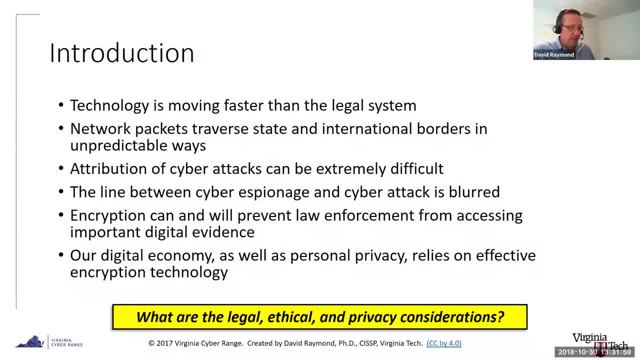 бы This crazy thing. There are obviously elections that are going on there right for like 80 percent of people And you know you've gotta be bit careful here to not just get all your data in your head. And so you know sort of turns in this debate where you know you point fingers to each other. But again this you have this. 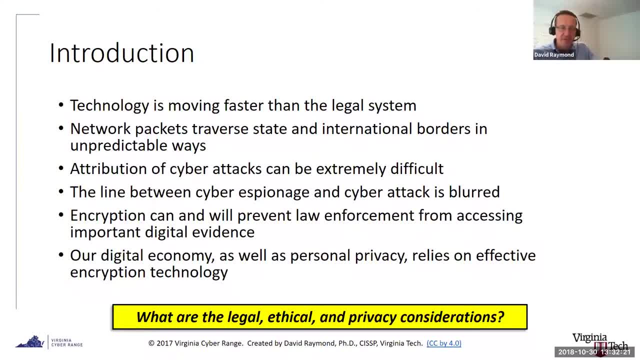 Unpredictable traffic routing and that can cause different issues. And then- so this takes us right to the third bullet- Right point the finger at China and say, hey, you purposely did this thing. And the Chinese say, no, we didn't, It was an accident, It was not malicious, It was a mistake. But it's hard to 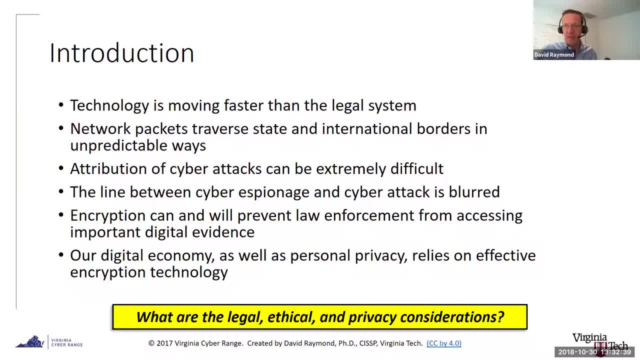 go back and prove that they did the wrong thing on purpose. But you know, the same is true with you know a bank gets hacked, for example, and there's always this investigation to try to tie that activity back to some individual or some- you know- group or some country. And it's not. 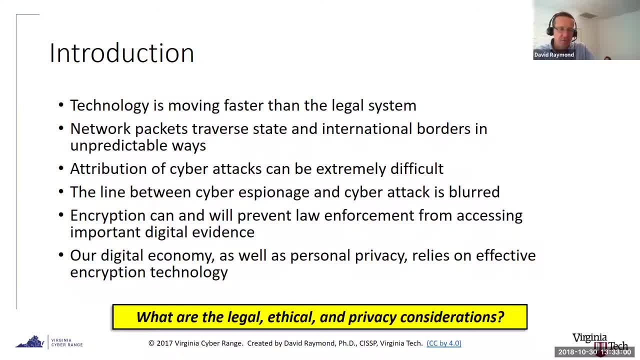 only extremely difficult. but it's also the case that many attackers will place essentially false evidence to misattribute cyber attacks right. So you know, maybe the Chinese will put in a bunch of Russian words in their malware, or you know, there's even cases where 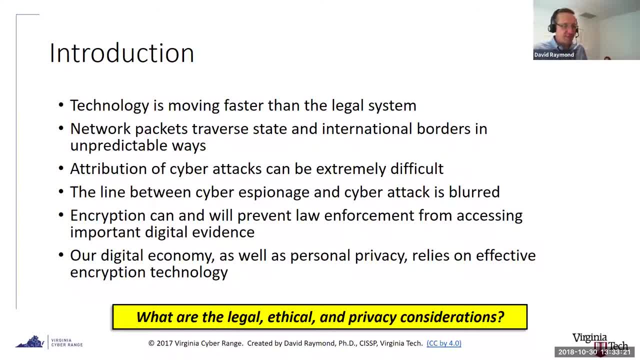 the Chinese will put in a bunch of Russian words in their malware. So you know, maybe the Chinese will put in a bunch of Russian words in their malware. So you know, maybe the Chinese will put in a bunch of Russian words in their malware. 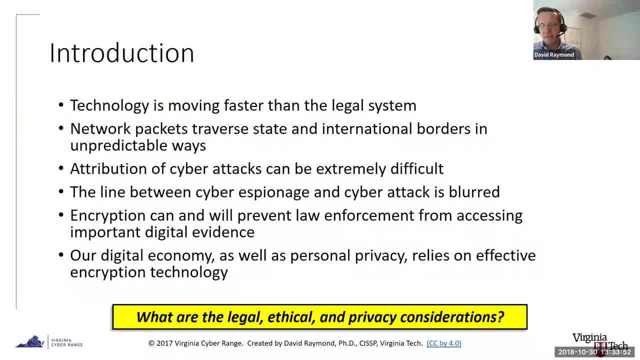 And there are companies that are actually very good at it. So CrowdStrike, for example, is a company that sort of you know. part of their business is based on very carefully attributing the parties that conduct different cyber security. you know different offensive. 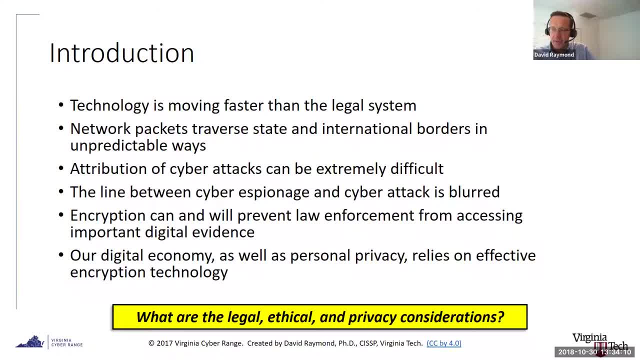 cyber operations, different hacking operations, But still, just because everybody sort of knows that attribution is so hard, even though you have a company that's very good at it and is usually you know, they can usually make the case very well. countries just sort of say, well, it wasn't. 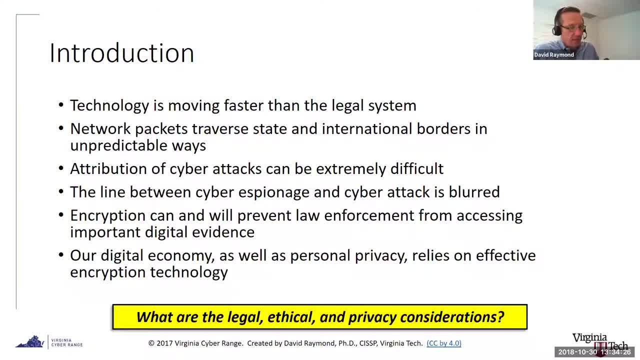 us And you know people say: well, you know the Chinese say it wasn't them. And we know that attribution is hard. So you know we'll never prove it to anybody's satisfaction. So that has effects on you know the ethics and laws of cyber security. Fourth bullet: there the line. 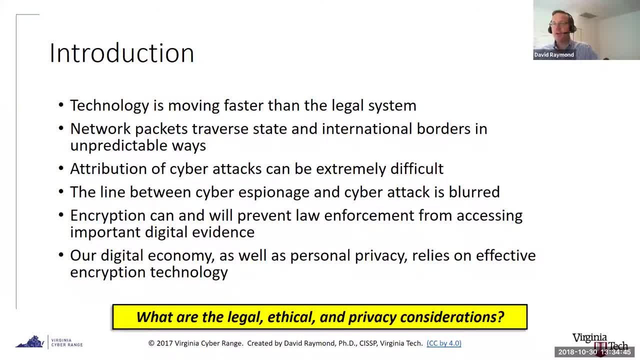 between cyber espionage and cyber attack is blurred. Okay, so what does that mean? Well, you know what. so we know what espionage and attack is, in sort of a you know, historical, international sense. Espionage is where you spy on other countries, governments or you know. 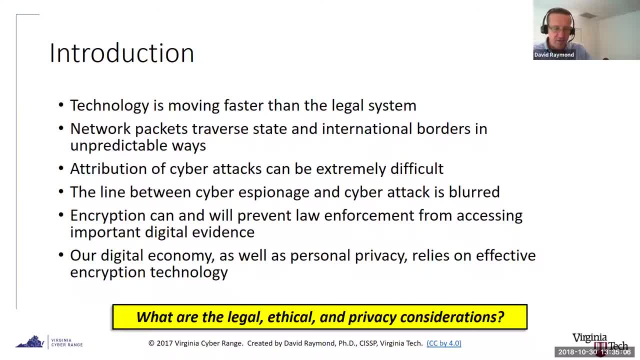 it's generally nation state spying on the activities of another nation state And you know the international law surrounding that is pretty nuanced, right. So there are some cases where you know some situations where espionage is clearly illegal. So if you're breaking and 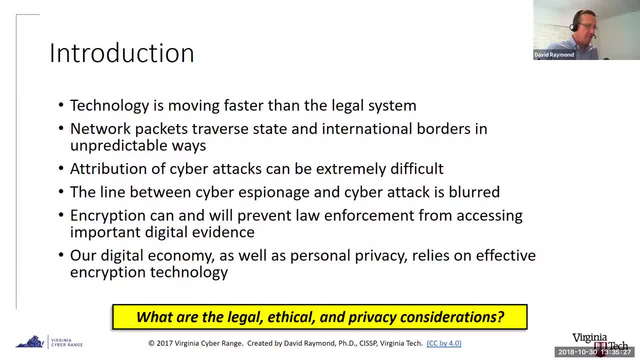 entering to conduct espionage, for example, that that's you know. you're violating some law somewhere. So you could point to that and say, well, this person is breaking the law, but some espionage is not illegal, It's you know. so if you're sitting outside in a cafe watching people, 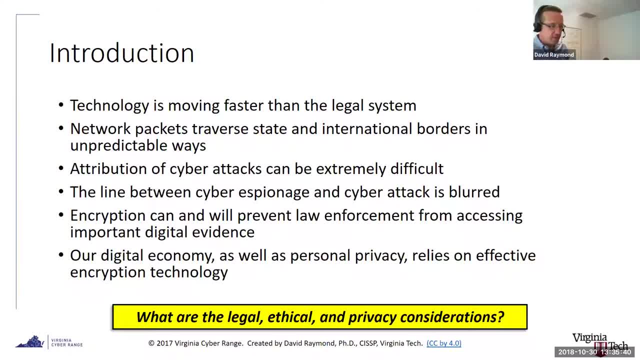 going in and out of the embassy and recording who goes in and out, when then you know there's no law being broken. That's sort of simple espionage, And so no harm, no foul, and countries do that to each other all the time. Cyber attack, on the other hand, is always wrong. I mean it's. 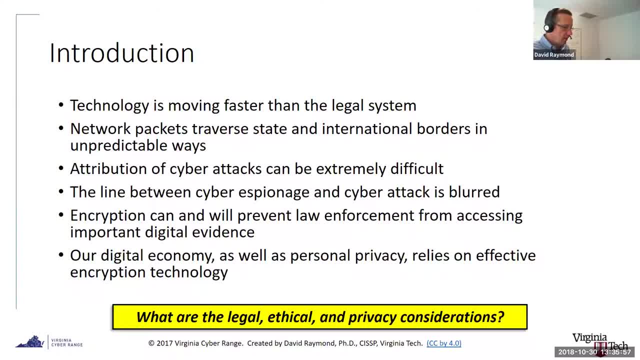 always wrong. maybe not always wrong, but it's always a violation of you know, if you attack somebody without provocation, that's always going to be a violation of international law And so and so now, if you get into cyberspace, what's what is espionage And what is cyber attack And a lot? 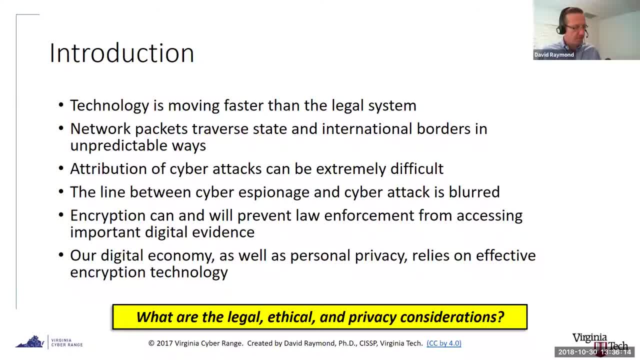 of a lot of nation state intelligence agencies conduct essentially offensive cybersecurity operations against other countries. they'll break into systems. they won't. they won't steal anything, you know. so they won't remove any intellectual property, they won't damage any data. they won't do anything except for eavesdrop on communications. 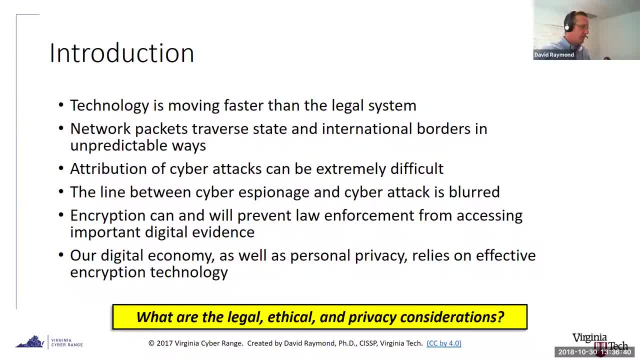 And you know they'll say that's just espionage And that's sort of become something that is that is recognized as espionage, And so countries do it all the time and they're sort of this understood. hey, we were just. you know we were, we were just spying on you. 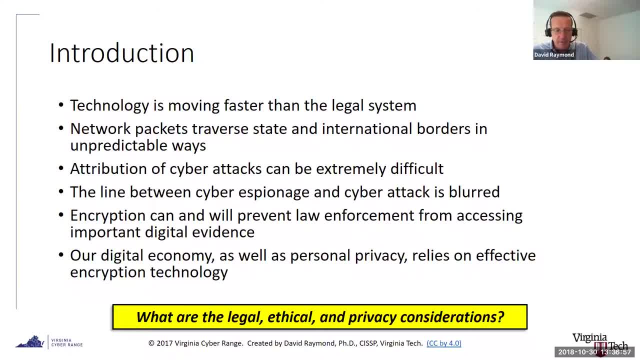 like we do, And so now we'll stop because we got caught and it doesn't turn into an international incident. The question is: where does the where's the line between espionage and attack? When is a? when is a one of these operations and attack, rather than just conducting espionage? And so if 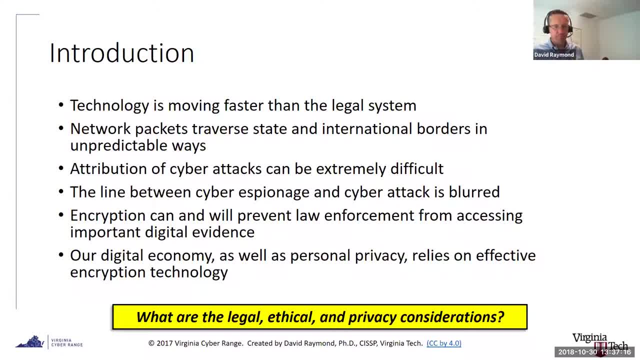 you think of the hacks, of the, of the, the DNC, that the Democratic National Convention email system in 2016,. you had all these. you know, you had all these emails, who were that were, that were taken, And then they were shared in different places to the. 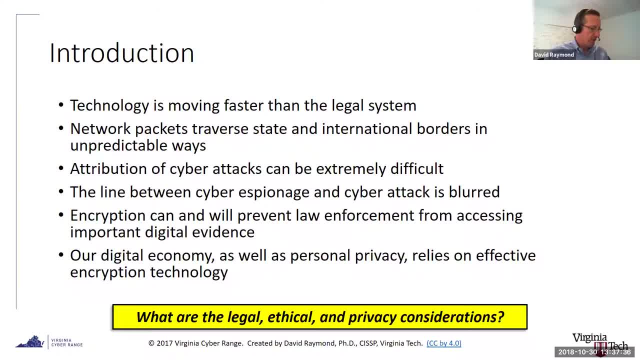 detriment of the Democratic National Party. And so you know, is that, did that cross the line between espionage and attack? You know again, this is, this is perhaps a situation where the laws haven't quite caught up, And so I don't know. I think that's useful to talk with students about. And then the last two bullets there are related to: 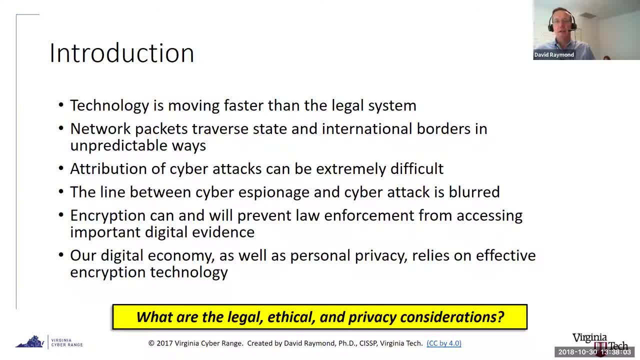 encryption. So the first one, or I should say the fifth bullet here: encryption can and will prevent law enforcement from accessing important digital evidence, And we will look at a case study related to that. Okay, so we've already seen this right. We've seen cases where people's cell phones, where people have conducted a crime, 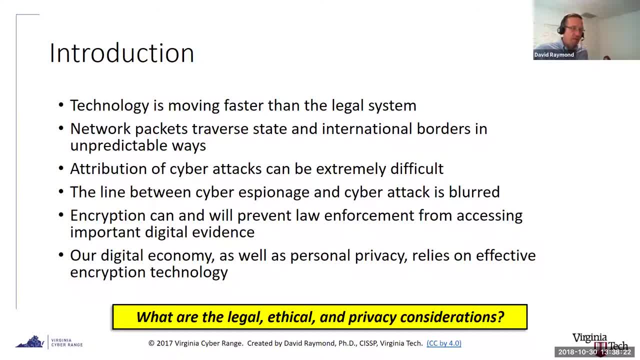 their cell phones have been locked and encrypted and law enforcement has asked for those cell phones to be to be decrypted so that they can- they can- review the data on the phone And and people have refused. And so now you can point to that. you can say: well, encryption is preventing law enforcement from doing its job properly. And we'll talk about a specific case study. 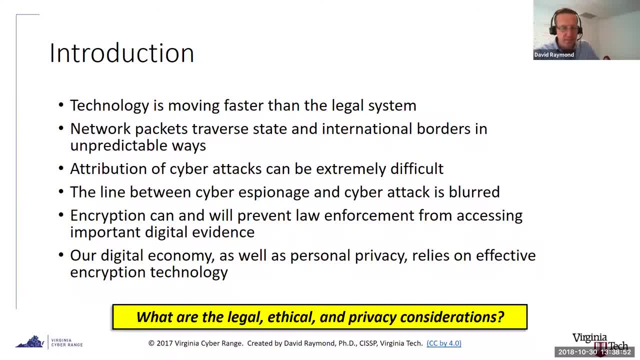 along those lines. Here's an interesting fact that most folks don't know: If you're, if your mobile device is encrypted. So if you have a passcode on your iPhone, for example, law enforcement cannot serve a warrant that requires you to put in your passcode to unlock the device, but they can serve you a warrant that requires you to use your thumbprint or other biometric to unlock the device, because 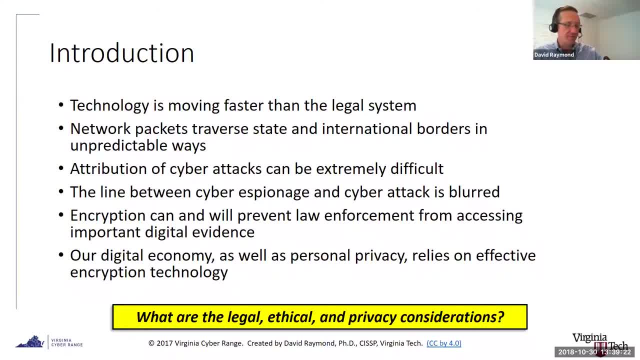 it basically comes down to knowledge versus a physical trait, right? So? so a search warrant can't require you to to give knowledge that could be self incriminating, like the four digit passcode on your phone, but they can force you to use your thumb to open the phone because 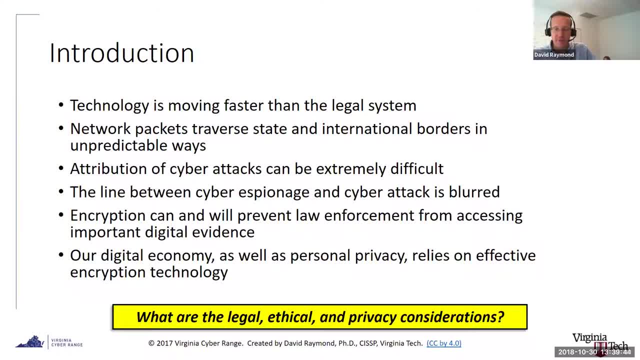 you're not imparting any knowledge that could be detrimental to your Fifth Amendment rights. Again, little known fact that a lot of folks don't- a lot of criminals don't know, which is probably good, but a lot of others don't know either. 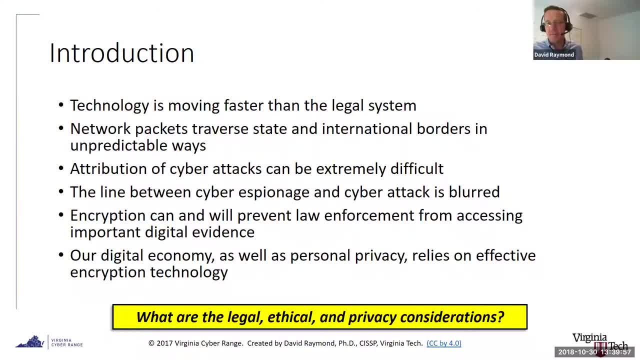 Okay, and then the last bullet. So this is. so the last bullet is is sort of in direct competition with the fifth bullet. right, Our digital economy, as well as personal privacy, relies on effective encryption technology. So on the one hand, we're saying that 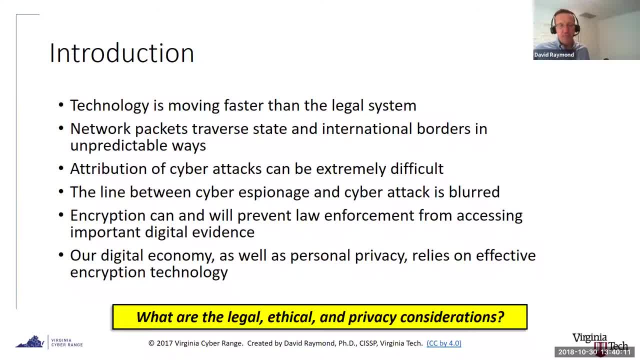 that our digital economy- I mean essentially the US banking system- is built on encryption. Without encryption, we could not have a digital banking system, And so that encryption needs to be as secure as we can possibly make it, or our economy could could suffer grave danger if there was some way to subvert it. 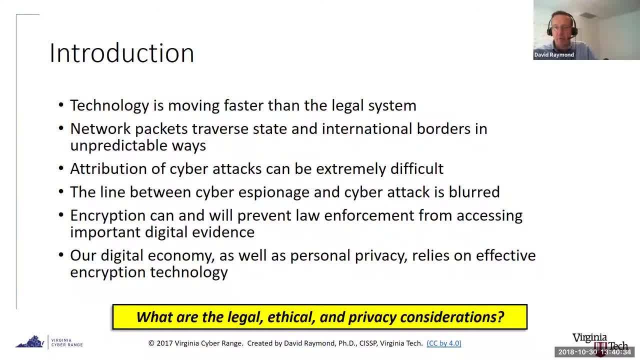 Okay, but on the other hand, we say that that great encryption that we use is used also in other instances that will prevent law enforcement from doing its job. And again we'll look at case studies that that rely on both of those. Okay, so let me dive into a couple of case studies. see how many I get to. First one here is Stuxnet. 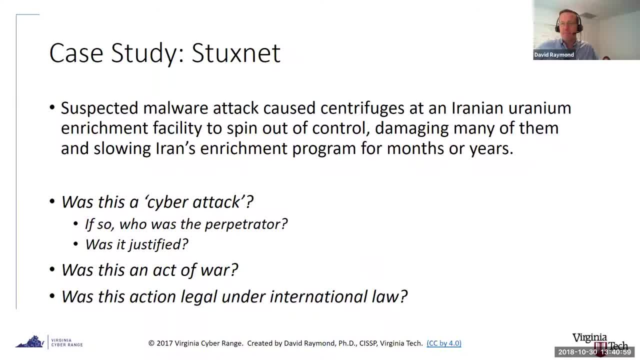 So this is so. Stuxnet is a piece of malware that, again, you know, the teachers will, you know, may remember this, Students probably won't, because it happened around 2010, but Stuxnet was malware. This is, this is really. 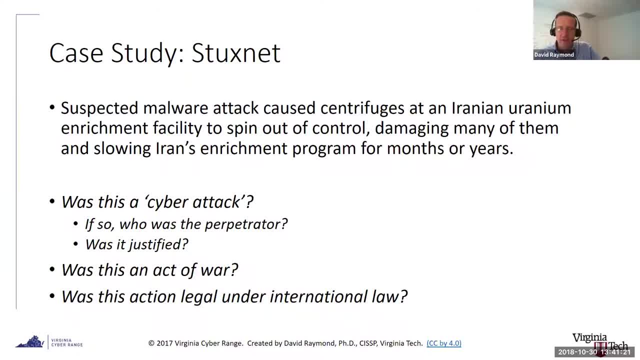 clever, actually, And there's a great book by Kim Zetter called Countdown to Zero Day. Type it in the chat here: Stuxnet, Stuxnet, Stuxnet. Book, Countdown to Zero Day by Kim Zetter. So this is a book about. it tells the whole story of Stuxnet, And there are other. 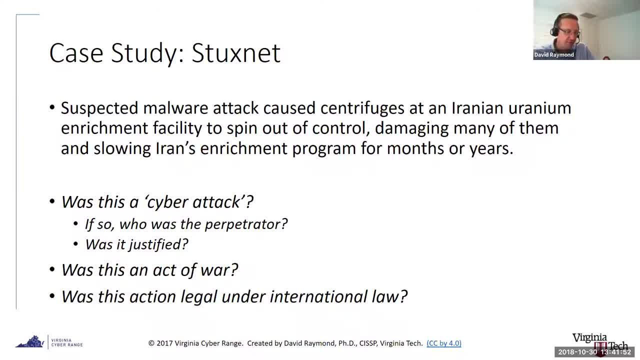 There's. there's some in the speaker notes for the slide. there's references to some other Stuxnet articles that sort of tell the story. Kim Zetter's discussion of it is really good. It's a. it's a book that sort of reads like a spy novel, but it's 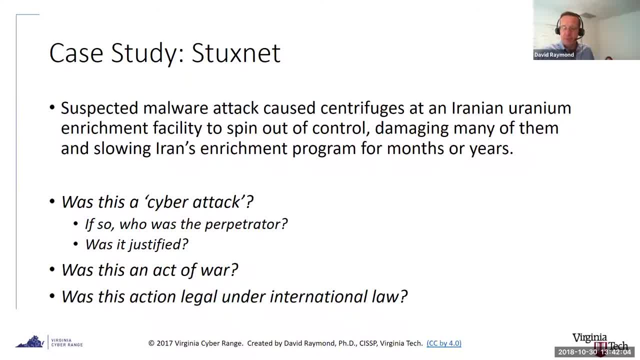 This was malware that was surreptitiously placed on centrifuges in an Iranian uranium enrichment facility. And what the what the malware did was? It was this multiple stage malware, right? So first, The first thing it did was it Very carefully identified exactly what type of systems it was running on. So it had all these checks to ensure that it was running on very specific, you know type of centrifuge with very specific control software and you know it was. it was all these tests to make sure that it couldn't. 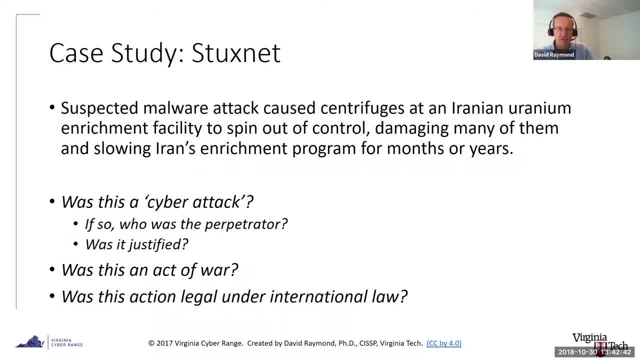 It couldn't execute the malicious payload unless it was on one of these centrifuges in this facility in Natanz In Iran. And So what? this whole series of checks, And then what it did, was it recorded the proper operation of the centrifuge for a long period of time, and then it started. 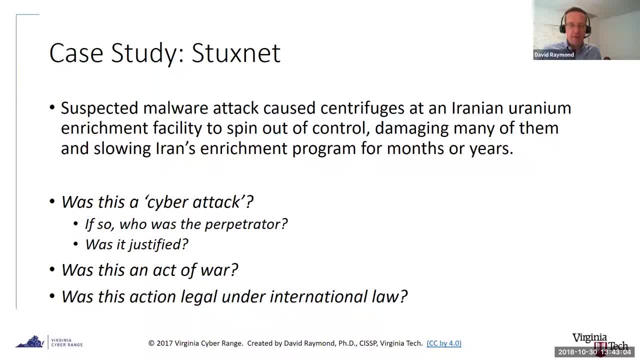 It started playing back, So it started Causing the centrifuges to spin faster and slower. So it would do this cycle where it would spin them too fast and spin them too slow, and spin them too fast and spin them too slow, but all the while it was taking this recorded proper operation and it was sending that to the 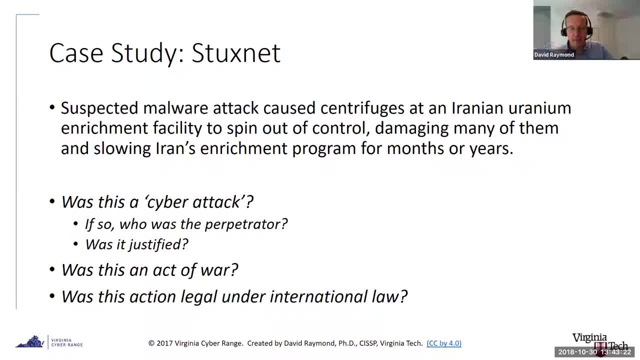 To the logging system so that it looked to the, to the. you know, outside this specific centrifuge looked like everything was operating normally, so that so the operators of the nuclear facility couldn't identify that these things are spinning out of control. but the But the centrifuges did this. 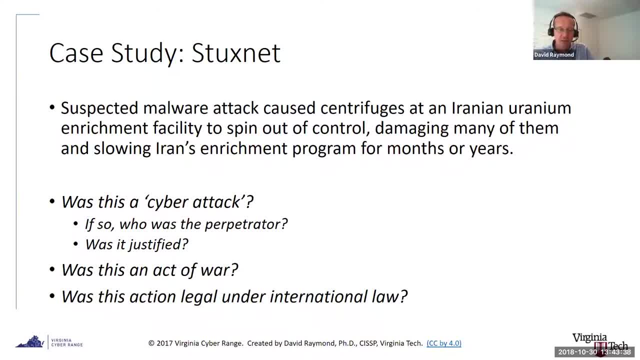 Crazy dance that essentially caused them to self destruct over time. you know, these are very finely tuned devices that need to operate a specific frequency, for, you know, for months to do the right thing, And if you Screw around with the way they operate, 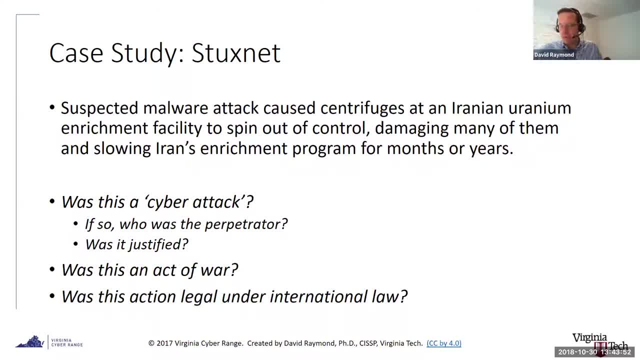 Then that You know that subverts that whole, that whole process, and it caused the cause, like thousands of these centrifuges, to basically self destruct and they and they traced it back to software that was Eventually traced back to the United States. actually, So it was. this was attributed to the United States. course, I mentioned that attribution is hard Right, So so I don't think anybody in the United States is as 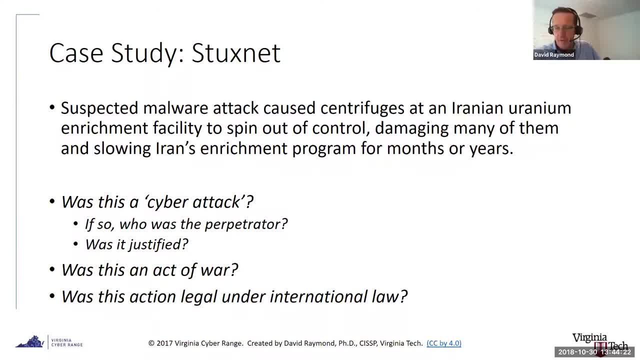 Sort of fessed up, but it was. but basically the National Security Agency was, was accused of doing this. And so here are some some questions for discussion. Right, Was this a cyber attack, You know? was this an act of war? I guess is, maybe is a better question. Was this an? was this an act of military aggression? and you know, there are specific, there's specific definitions that go along with that definition of an act of war and basically, 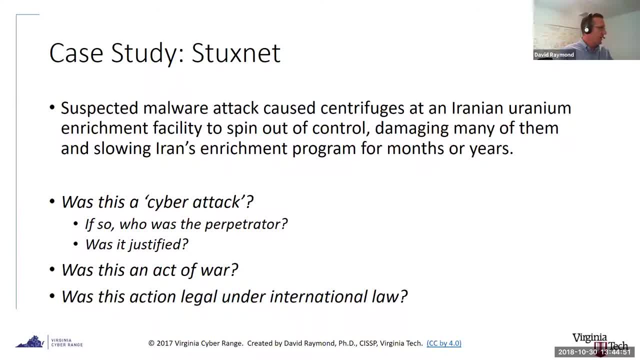 You know, we say that An act of war must be an action that kills people or breaks things right. so if it doesn't kill people or break things, then it's not an act of war. So so these sort of routine attacks on the DNC, for example. so you know, cyber attack. 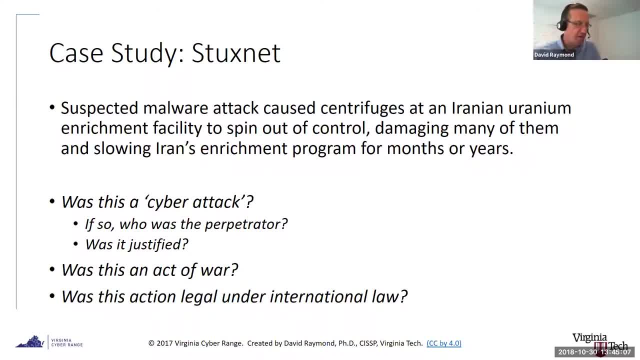 Reportedly by Russia against the DNC Democratic National Committee. you know people. some people would point to that and say: oh it's they're. they're violating our election system And that's an act of war, And I think just about everybody. 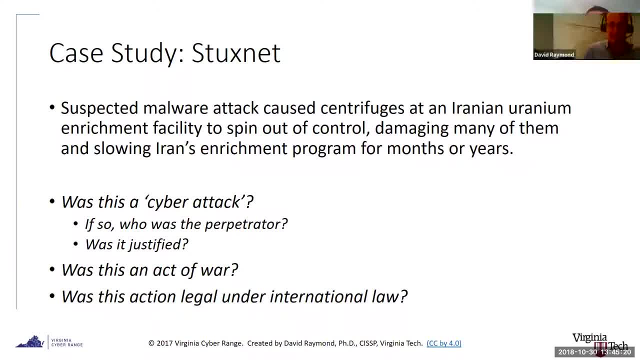 Just about every international legal scholar would say that's not an act of war, That's that's. You know, that's certainly an exaggeration, But in this case these things were damaged, right, these centrifuges were damaged, And so You could classify this as an act of war against by the United States against Iran. Some people would would classify it as such. 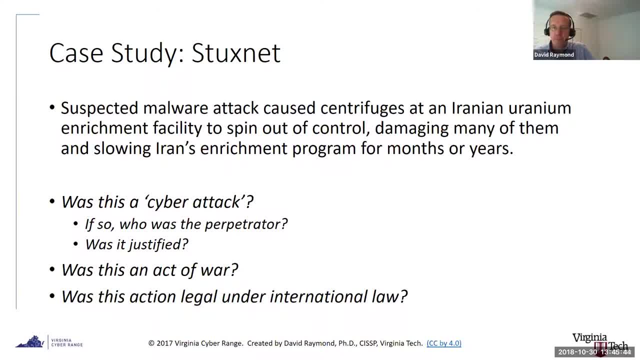 And then You know: so, was this action legal under international law? Under international law, Is this something that You know? is this something that that, if the United States was responsible, should they be punished for it? And then you could get into a separate discussion about is. was this an ethical you know? was this a? was this a justified? 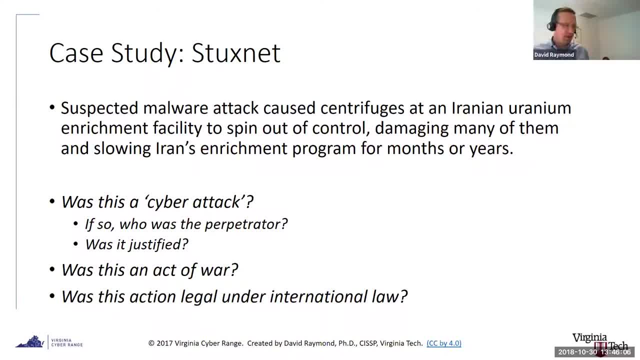 Attack. you know what, what was the, what was the purpose of the facility? What was the motives of the Iranians? and was this, was this: if this wasn't an act of war, Was it justified? You know, and you can sort of get into the 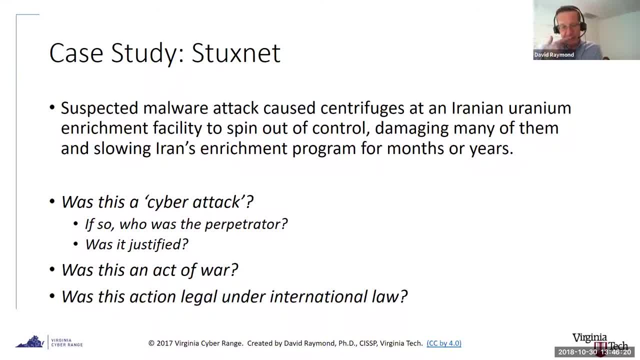 moral, ethical discussion with your students, And you know this is one of those things where there's really no, there's really no real answer, correct answer. you know you might come to a conclusion as a class, or or you might At least have a have an interesting debate about, about. 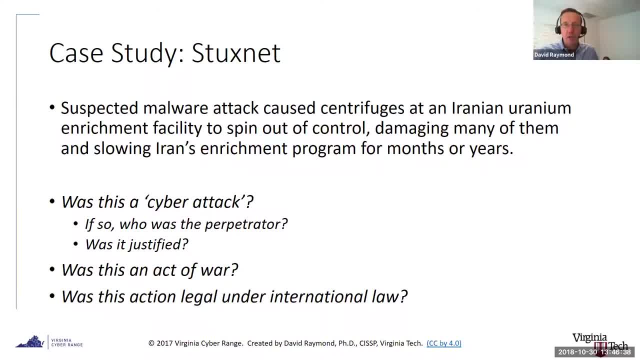 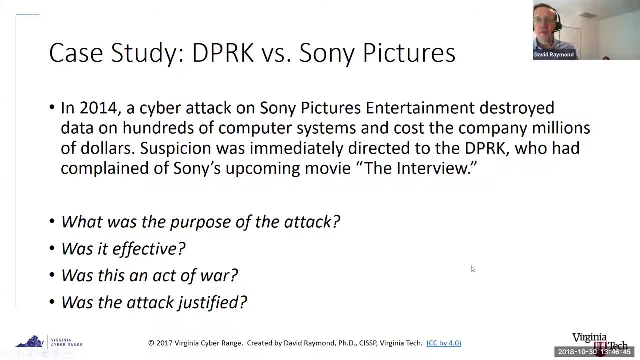 You know motives and who was right and who's wrong. Okay, let me dive into Another one here: DPRK- people's republic of korea versus sony pictures. this is a little bit more recent. 2014 um, a cyber attack on sony pictures entertainment destroyed data on hundreds of computer systems and cost the 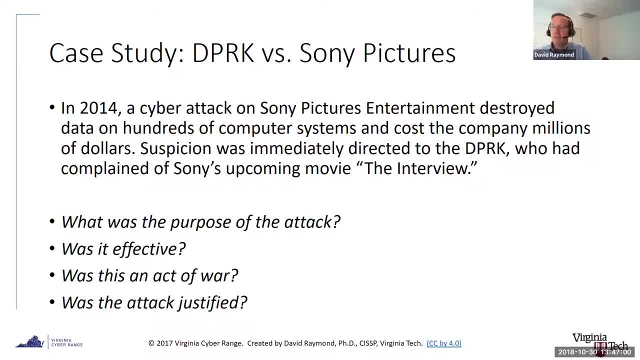 company millions of dollars. suspicion was immediately directed to uh, north korea, who had complained of sony's upcoming movie, the interview. so this is a movie about, um, a couple of goofballs who were sent to north korea or i don't know. i guess they were going there to 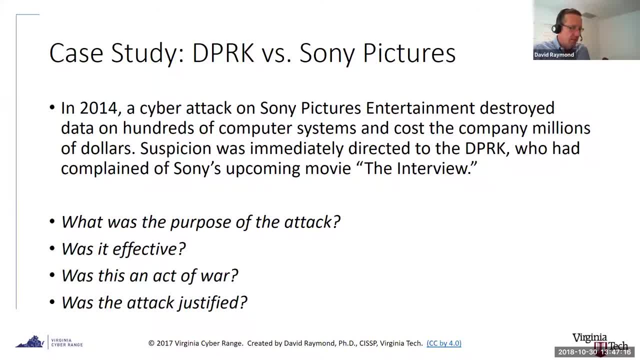 film, a show or something, and you know, this whole thing's supposed to be a comedy, and and they um were uh recruited by the us government to to kill um kim jong-un, and this was you know. of course, the north koreans saw this as a you know sort of blatant um slap in the face. 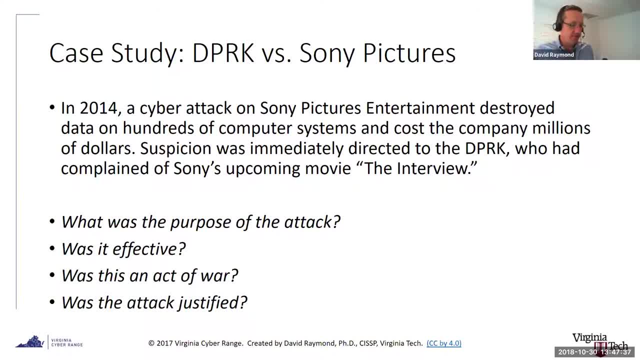 and they warned: uh, sony, that if you know they, they, this movie was released, there'd be grave consequences and etc. etc. you And the movie was released anyway and the North Koreans attacked. This is pretty well attributed to the North Koreans. They hacked Sony Pictures Entertainment and cost the company millions of dollars in damages. 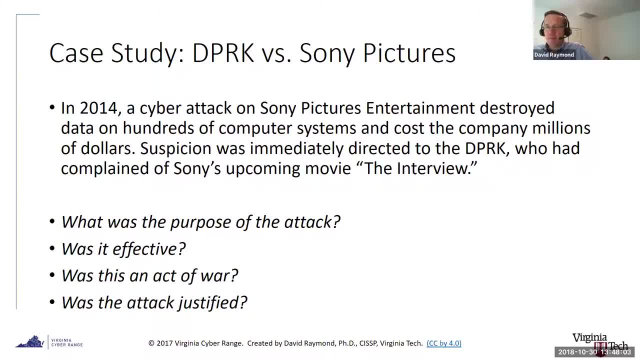 And so then you can have the same sort of discussion, right. What was the purpose of the attack? Was it effective, Was it an act of war, Was it justified? And I think you could probably say that, you know, in the end it probably benefited Sony, because I think the interview was a bad movie or it wasn't a movie that was going to do very well at the box office. 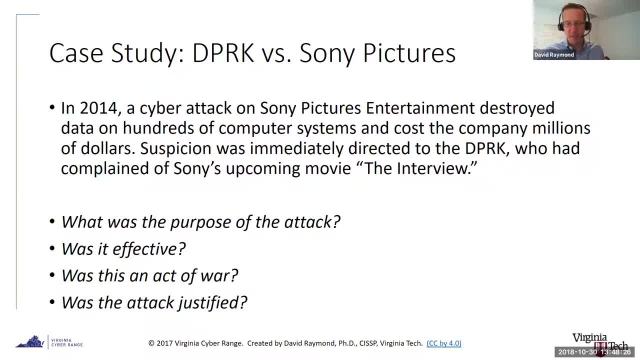 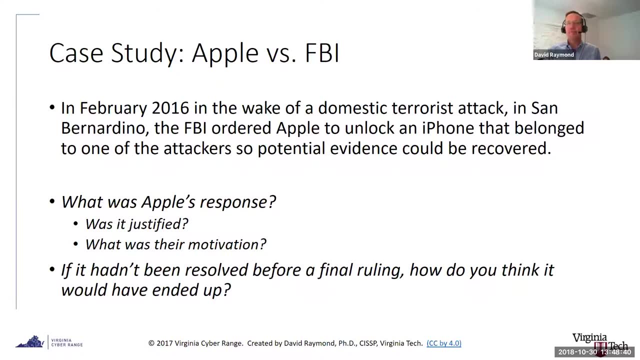 But the fact that this happened. I mean they probably made their money back in droves because people wanted to see it, just to see what all the excitement was about. Anyway, worth discussing with students. This, maybe, is even a better one. February 2016,. in the wake of a domestic terrorist attack in San Bernardino, the FBI ordered Apple to unlock an iPhone that belonged to one of the attackers so that potential evidence could be recovered. 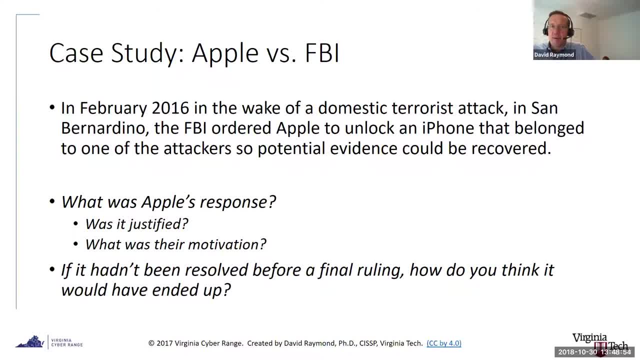 And you know, you teachers probably remember this well. So this 2016,, so just a couple of years ago, two and a half years ago, I guess. And so what did Apple do? FBI asked Apple to unlock the iPhone. 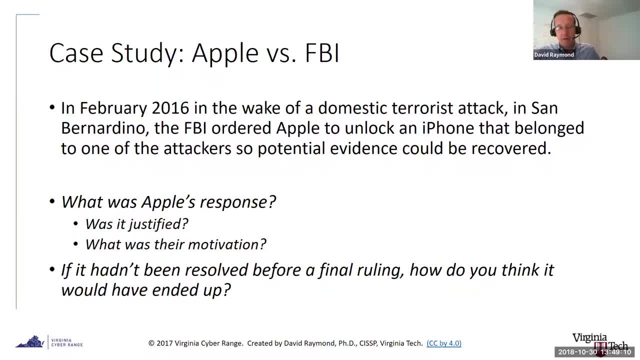 What did Apple do? Well, they said no, we're not going to do it, And that's what caused the news right, The fact that they asked Apple to do it was not news. In fact, here's another of those, you know, little known pieces of data. 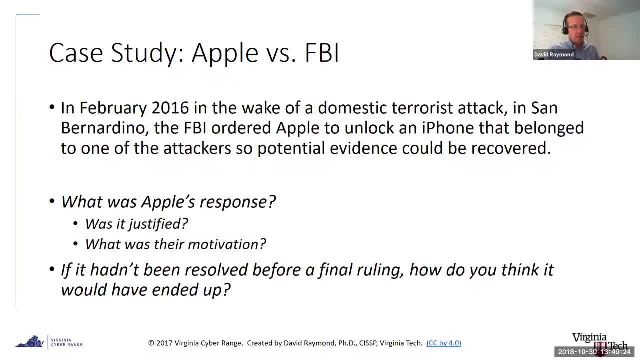 The fact is that Apple had done this multiple times before They had unlocked. you know. they had been asked by the FBI to unlock phones and they had done it and given the data over to the FBI, But in this case they refused. 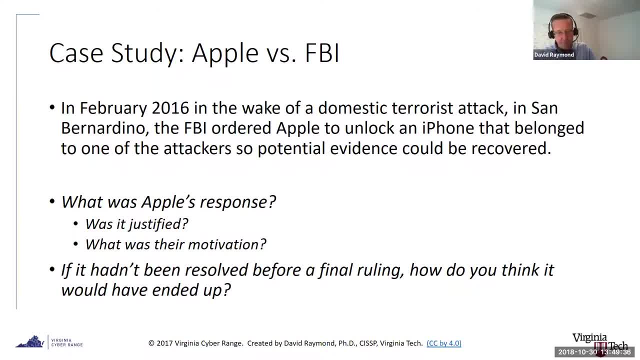 And so that's a that's a interesting fact to throw out to the students. OK, Apple had done this before. All of a sudden they say no. Why did they say no? What was their motivation? Right, And so some people who are cynical might say: well, Apple just did that because they wanted the press out of it. 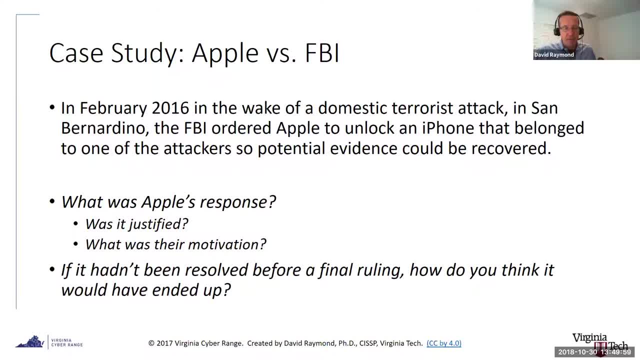 They wanted to be able to say: we protect our users data, even if those users could be, you know, evil or whatever. So that's how much you can trust us to protect your data. That's what cynics would say, And there's a lot of cynics in this case. 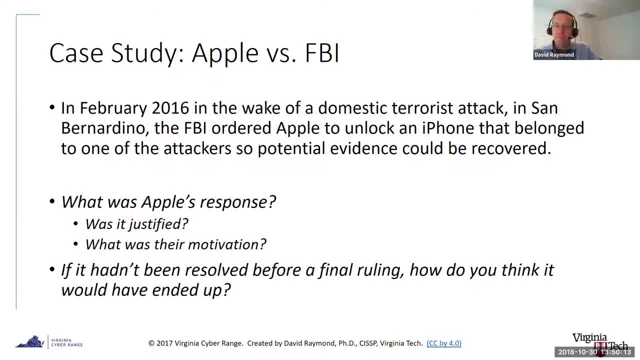 So that's worth talking about. And actually, if you continue the thread, what happens is Apple refused to unlock the iPhone for what they said were technical reasons and privacy reasons. Turns out that the FBI essentially hired a third party company to unlock the iPhone and they got the data off the phone. 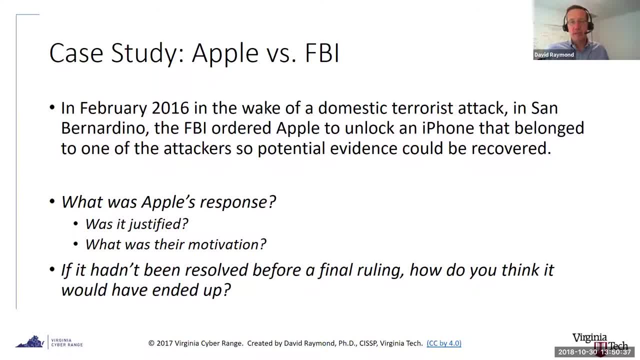 And? but you know the question is The second major bullet there, the third major bullet there: if, if, if this situation hadn't been resolved before a final ruling- So you know, the data was recovered and given to the FBI before, before there's a final court decision that said Apple, you need to do it, or not? 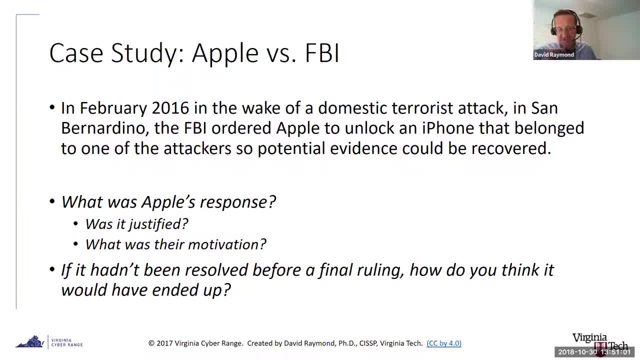 And you know. so the question here is: you know if this, if this hadn't been resolved before that court decision was made? And here's a case where the FBI gets to decide that you know it's okay with it by the theatricalide? 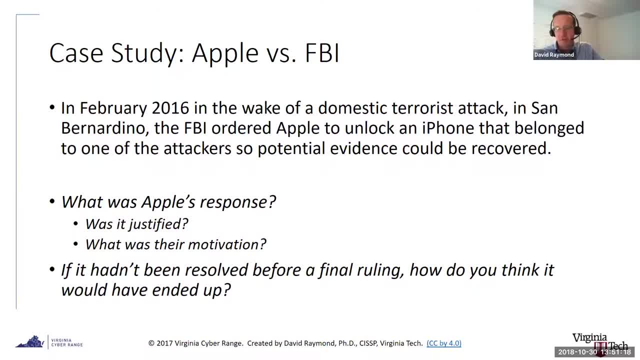 And here's the third reason. So in this case, where do we think this would have ended up? What would Apple have been required to do this thing, or what they have been able to fight off the legal action? So this is a case where you have encryption technology that is potentially preventing law enforcement from doing its job. 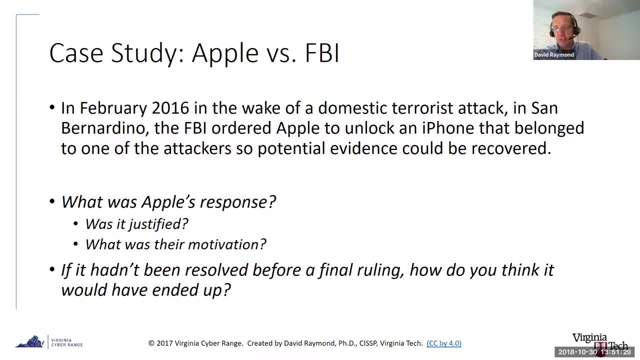 And Apple will say: they don't have a master key, right, There's no master key that they get to use. And they're right, there isn't a master key. and there shouldn't be a master key because, if there was, what happens? if? 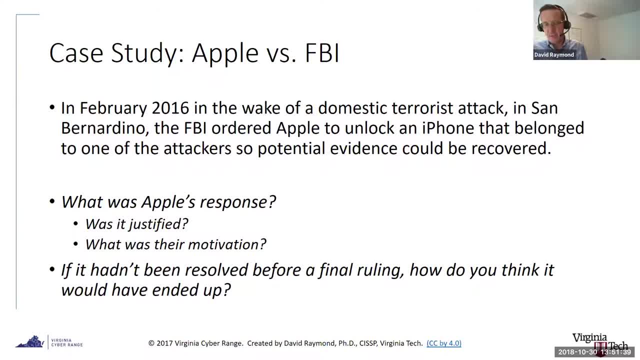 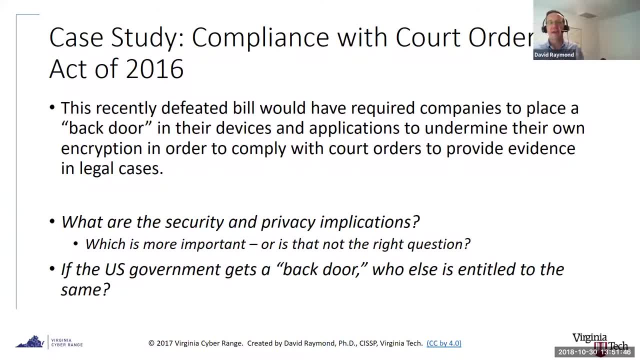 that master key got in the wrong hands, then everybody's data would be, could potentially be disclosed. so this follows right on that same thread: compliance. this is a- this is a law that was proposed in 2016, the compliance with court orders act of 2016. so this is this- was defeated. 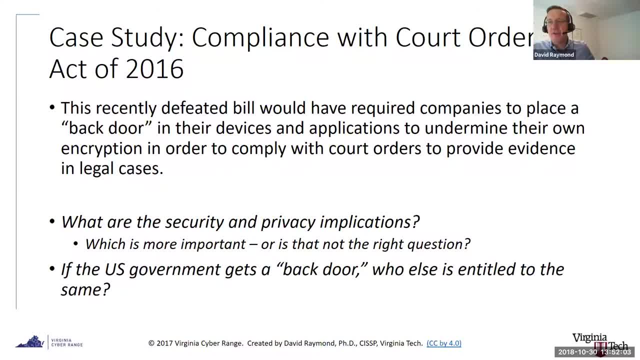 in 2016, but it was a bill that would have required companies to place a backdoor in their devices and applications to undermine their own encryption in order to comply with court orders to provide evidence in legal cases. so, basically, this is. this was legislators who said. 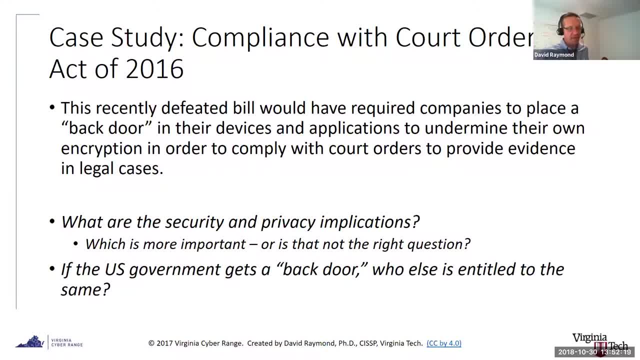 okay, apple, and your and your friends who make encryption- you know who make devices that have encryption- we're going to force you to put in a backdoor so that if law enforcement asks for the, for the um, for the data off the devices you have, you will. 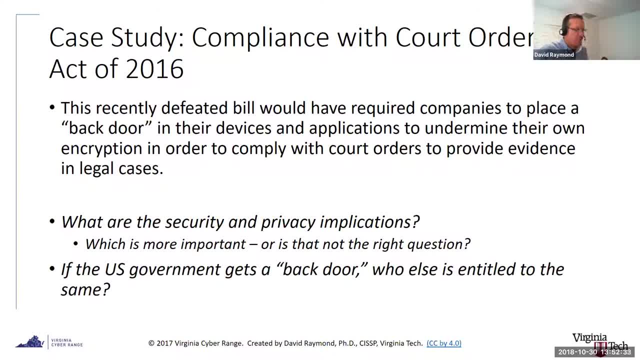 have a way to, to give it to them and, um, of course, from, from, from, uh, the privacy side of things, there i mean a huge uproar, right? um, you know, you can't, you know, the question is, um, you know, so the my second bullet there, uh, the first hyphenated or the first italicized bullet. 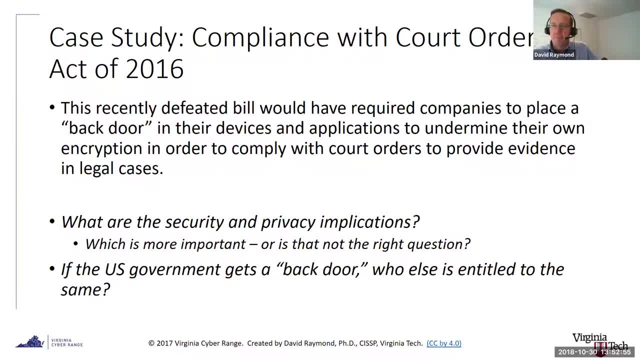 what are the security and privacy implications? um, and it's, it almost gets down to, which is more important. is security more important or is privacy more important? or is that not even the right question, right? so you know, on the privacy side, you say, well, if you're going to provide privacy, you have to. you can't put in a backdoor. well, if 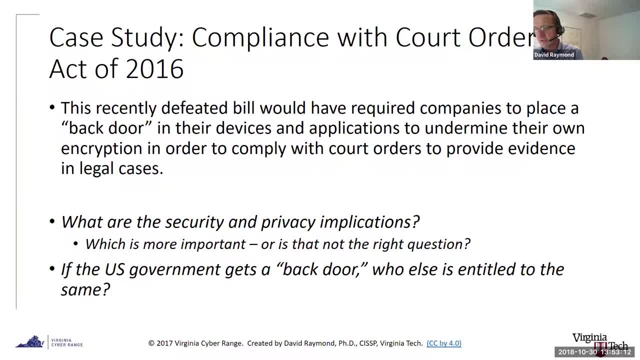 you want to provide security, you have to provide in a backdoor because you have to be able to- um, you have to be able to provide law enforcement with this data. then i'm not going to be able to secure people from future malicious acts that use encryption technologies to hide. 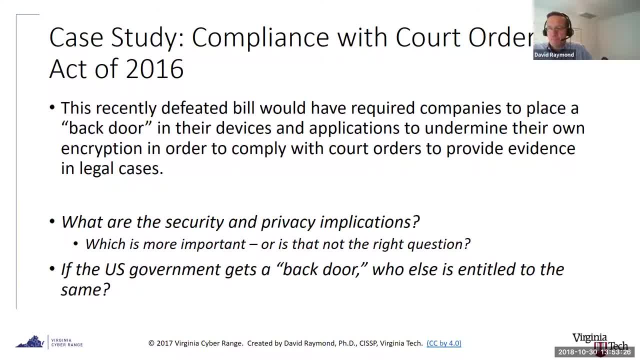 activities of malicious people. um, but then you get into some deeper questions about. you know this was: this could only be applied to us technologies, right? so? so this couldn't be um required of companies in other countries, who who write software or who produce um mobile devices that have encryption on them? so, um, so then the question: 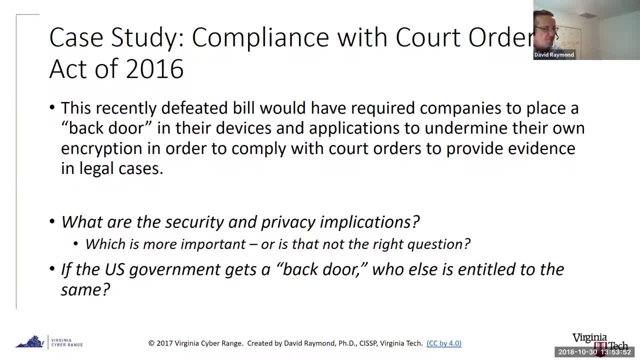 is, if us companies are forced to put back doors into the encryption, then what's going to happen to the market value of those companies? and i think what you'd realize quickly is that nobody's going to buy a us cell phone anymore. if they're, if they know that there's a backdoor in the. 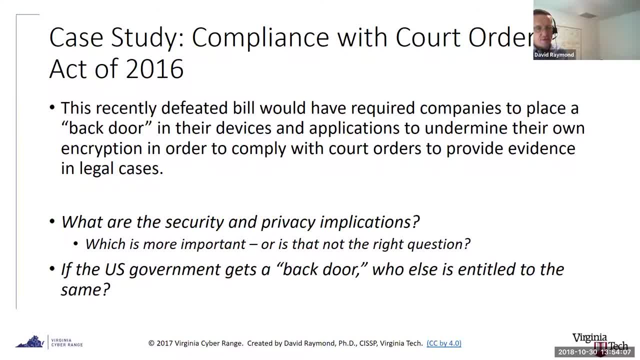 encryption because they can't trust it to be private, and so they're. so those companies essentially go out of business, um, and maybe that's a good thing, i mean, you know so. so, um, then another question is: so if the us government says, hey, all you companies, you need to provide a 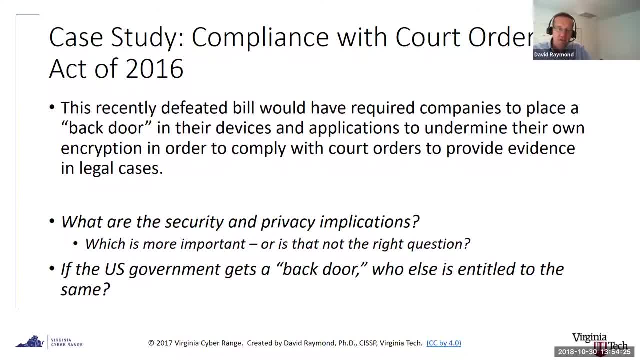 backdoor so that we can get in. what? what happens if, um, you know, do we share that backdoor with our allies? you know, i think an ally could could say: hey, we deserve to have that information as well. we should have the backdoor so that we can get in in case somebody in germany uses an iphone and commits a. 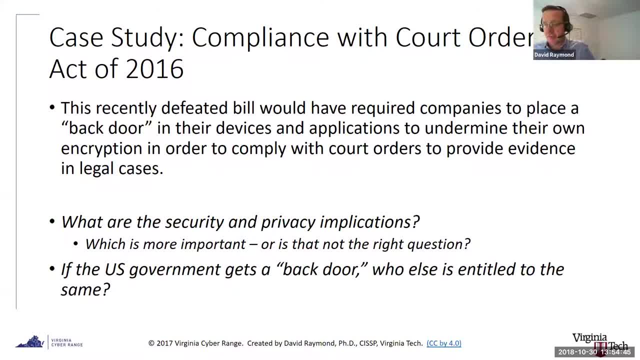 crime and we want to trace their uh, online activity, for example. and then, okay, so now we provide it to the us government and we provide it to the, to the allies of the us government. what about our adversaries? you know what? if? what if? um iran says, hey, we have crime too in our country and we want 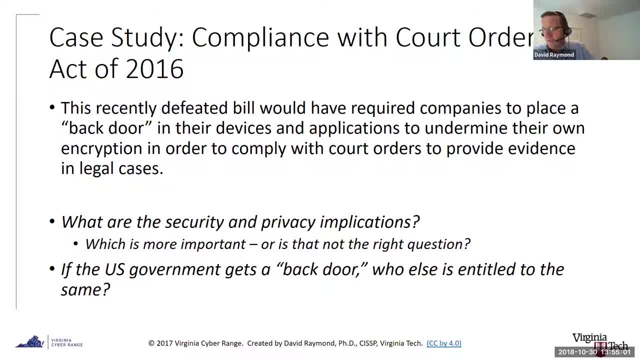 to trace back malicious activity and we want to trace back malicious activity and we want to trace back malicious activity on uh mobile devices. so we should get the backdoor so that we can use it on our, on people in our country and, um, i don't know, you sort of go down this rabbit hole, i think. 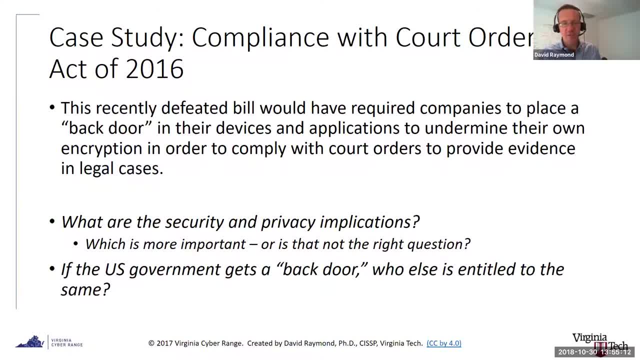 the, the um. it's an interesting discussion, i think you know. personal opinion is that the backdoor thing is is a broken concept. it'll never fly um. and again it comes back to the fact that our digital economy is reliant on secure encryption systems and any backdoor that you place in. 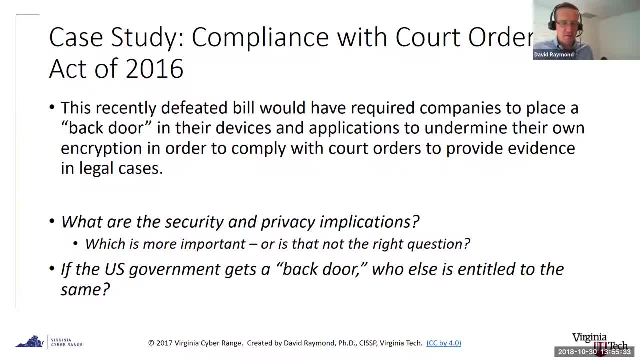 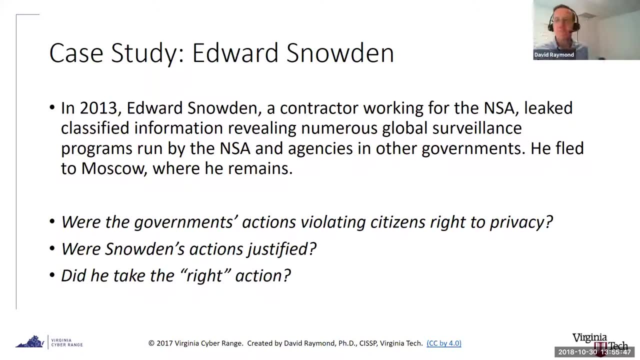 the back of your device. you're not going to get a hold of it. and then you know, once, once that, um, pandora's box is open, then you're, you're pretty much, uh, you know, out of luck after that, okay, um, uh, edwards, this is, this is the last case study, i think. um, this is something. again, teachers will. 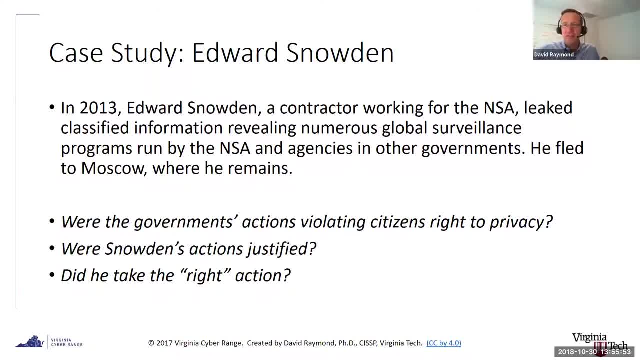 remember 2013. edward snowden, a contractor working for the for the nsa, leaked classified information revealing numerous global surveillance programs run by the nsa and agencies and other governments. uh, he fled to moscow, where he remains, so he's he's now living in moscow, um. 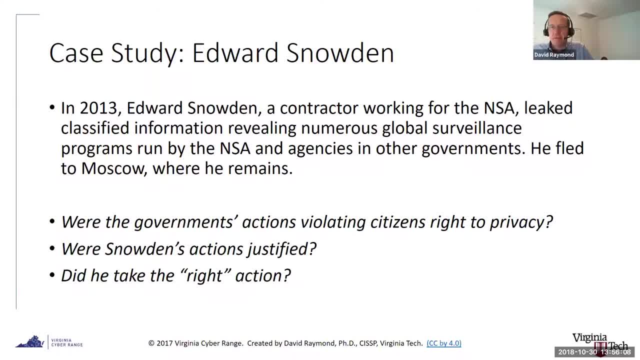 and so here here are questions: were so um? were the government's actions violating citizens right to privacy? so there are these. i mean, if you look at some of these documents there was, there was sort of this: this wide scale um eavesdropping on uh cellular telephone calls and the. you know this. 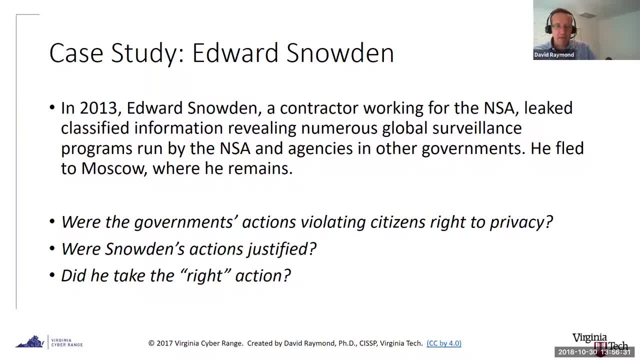 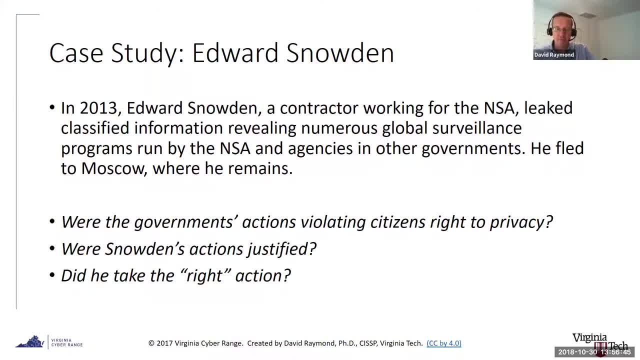 activity that we suspect later on, then we can. then we can go listen to those cell phone calls and see what they were talking about, for example. but i mean there's some, there's some, definitely some things in the edward snowden files that privacy advocates would say, hey, this is a clear. 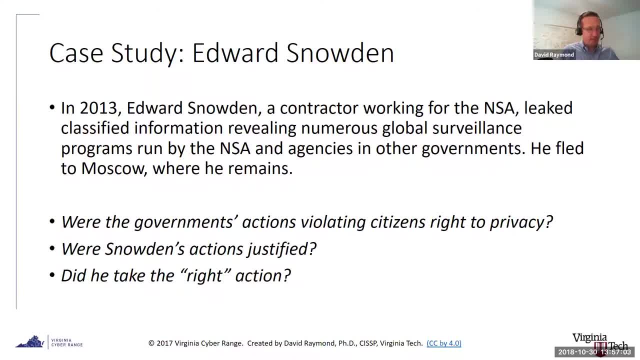 um, and you know the question, and i mean this might, that might even be interesting to sort of dig some of these documents up and and see what was disclosed, because i think you'll, i think it won't be hard for you to show the students, hey, look this, this, look, this kind of smells. funny, you know. 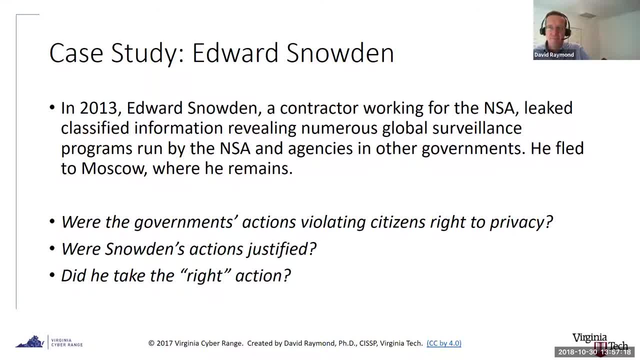 the some of the data that was being uh, um, that was being captured by uh intelligence agencies in the us and um. so the questions here were: the government's actions violating citizens right to privacy? um, you know, were stonings? were snowden's actions justified? so, snowden, he was a contractor. 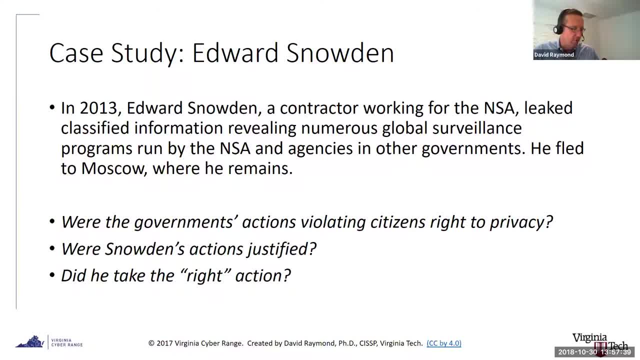 he wasn't an employee. he's simply a contractor working for an intelligence agency, an agency, and he, um you know, basically smuggled these documents out and shared them with news media organizations. you know, was was what he did justified. i mean, what? what other action could he have taken? did? 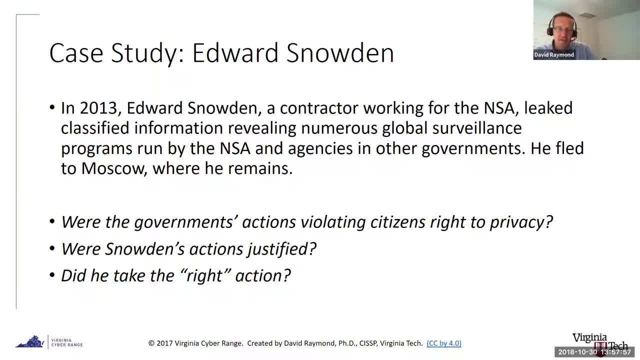 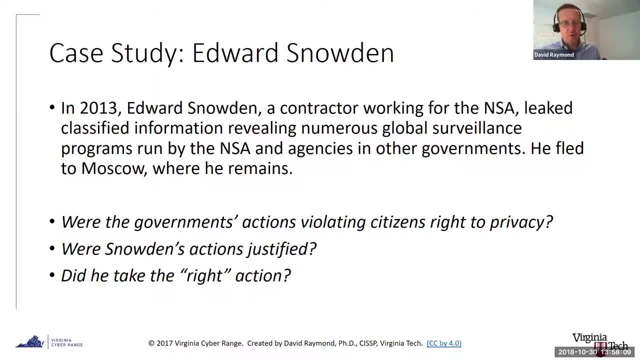 this is a thing where you- i think, um, you know most students sort of quickly go down this path that they say: hey, you know, these things were egregious, you know, the intelligence agencies were were eavesdropping on on private interactions between individual citizens who are not suspected. 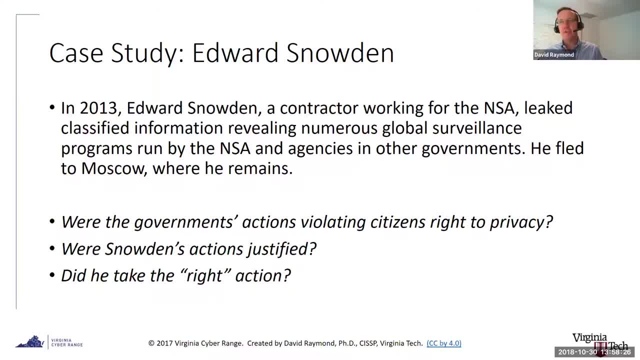 of committing any crime and, um, clearly a violation. okay, but then if you put this in context, you think back to um, september 11th. right, what happened after september 11th? and again, this that's. you know, the students aren't going to remember this, but the teachers probably will. 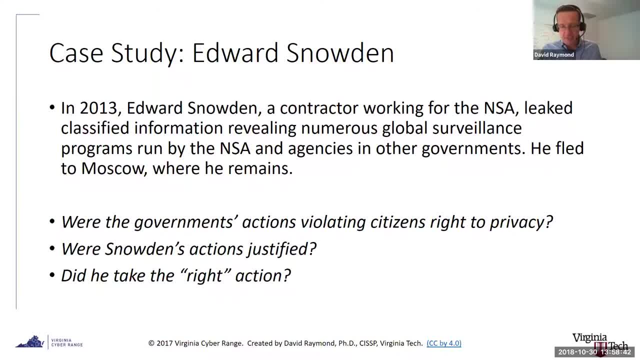 um, you know, these, these intelligence agencies were. i mean, they were raked over the coals, right they were. they were told in no uncertain terms by the congress of the united states that you better figure out a way to prevent something like this from happening again, right? 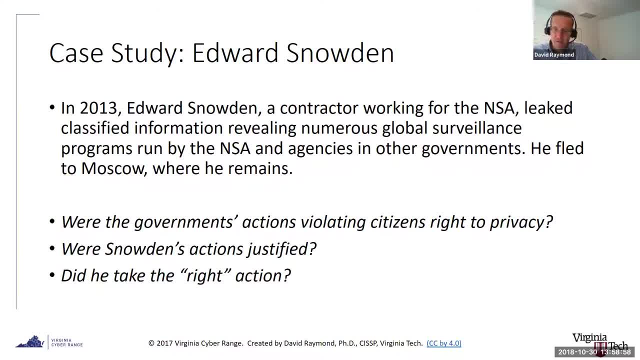 the congress said: hey, you know that september 11th that should have been predicted by us intelligence agencies. how could you not have seen this coming? how could this happen with the technology that's available to you at this day and age? and, by god, you better. 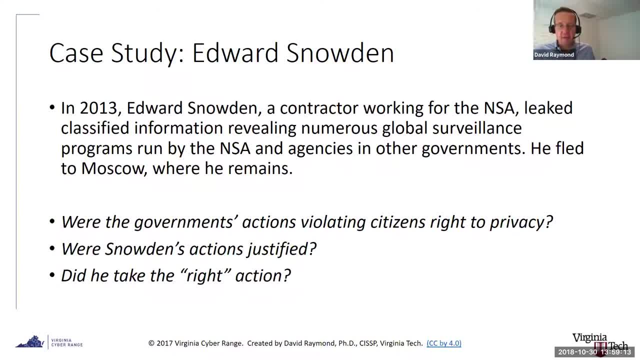 figure out a way to stop it from happening again. and you know, so that's the, that's the context under which these different surveillance programs were were created. and, um, you know, even after the snowden documents, you had a lot of lawmakers who sort of pointed back to. you know, 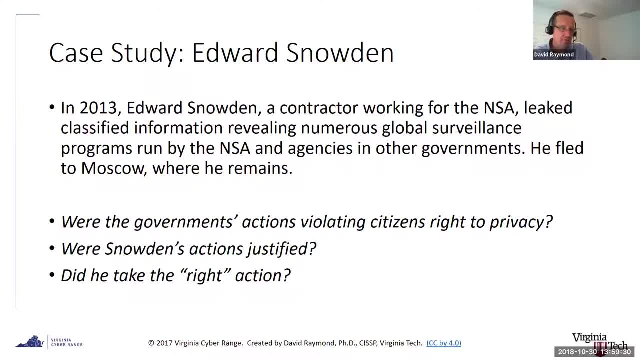 pointed to the the snowden documents and said: hey, you know, of course this is a violation and and the nsa should be ashamed. but really, um, you know, these are the same lawmakers who who rake the nsa over the coals after september 11th. so, you know, that's the kind of thing that's, that sort of gets both sides of. 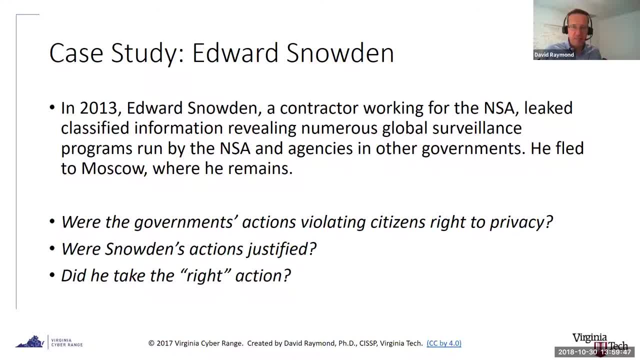 the argument and- and you know, this is the- this is the kind of a case study where you might, you know, assign it to groups of students and say, hey, you know, some have. you know, this group take pro, this group take con, and we'll debate it right, talk about what we think is right and what, what we 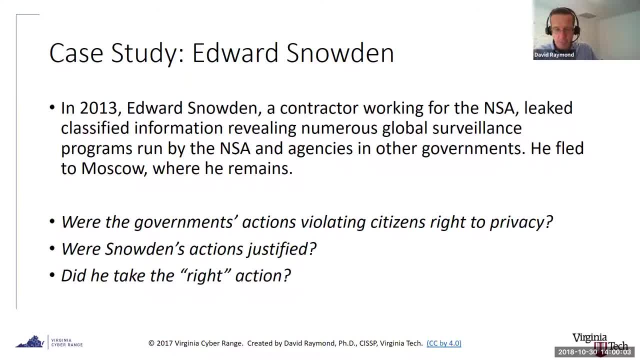 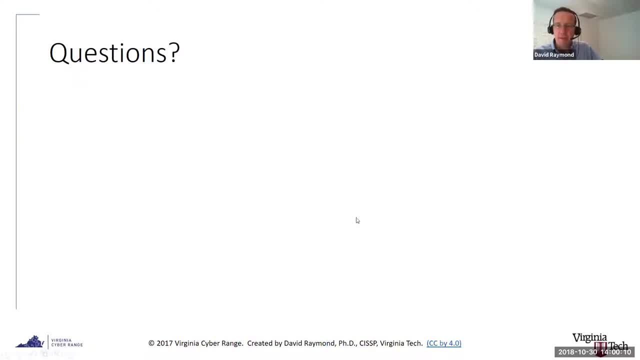 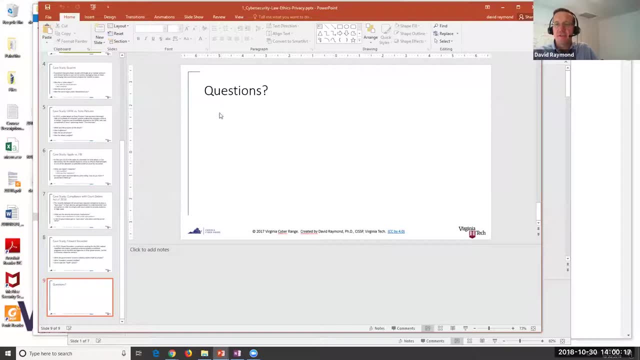 think um, so anyway, interesting case study, i think okay, so, um, so that. so these are obviously much better if there's um, you know, if you have students in a room and you can sort of get this discussion uh going um, and i would also suggest that maybe you um look at some other um, you know so a lot. 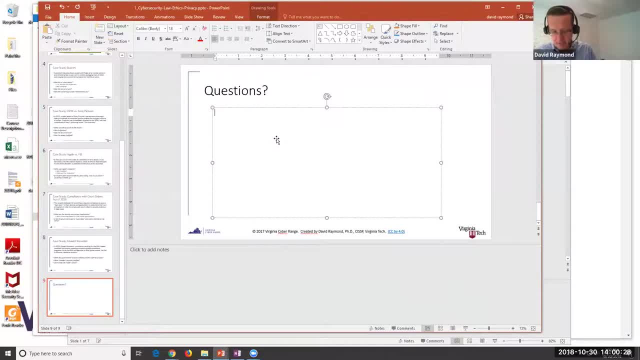 of these are sort of politicized and maybe pretty deep for a bunch of high school kids. um, you might look at uh, some other technologies and think of the ethical implications. uh, things like uh self driving cars, for example. um, make this a little bigger so you can see it: self-driving cars- you. 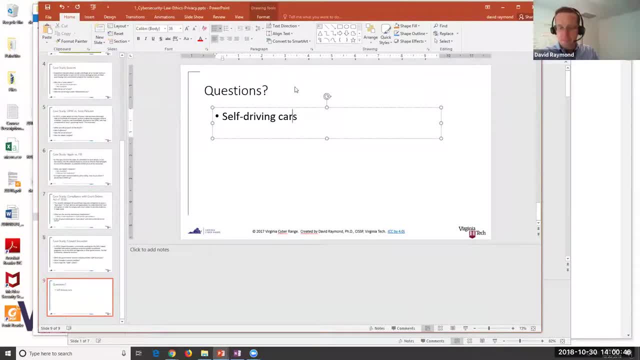 might have a, you might have a discussion about. you know what are the, what are the um implications, uh, um ethical and otherwise from from that uh drone technology right. so now we have all these. you know you. you know, 10 years ago um drones were uh very much a hobby activity. in fact, you know remote control aircraft- aircraft have been a. 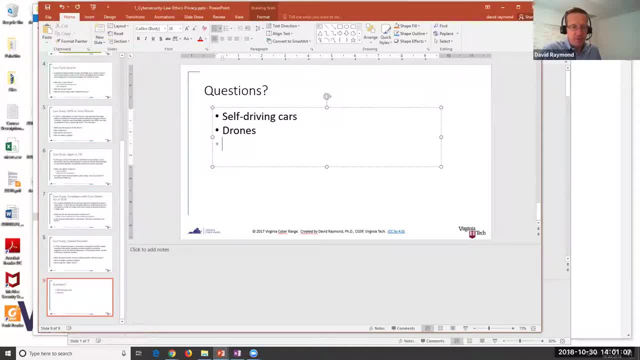 hobby activity for you know, 100 years, almost, um. but now you have. now anybody can go to walmart and buy a drone for 50 bucks, and now they can be flying this thing with a camera on it around other people's homes. and so what you know? how should they be regulated? should they be regulated? 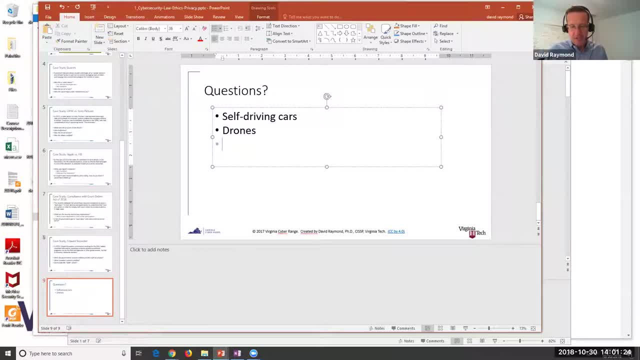 um, you know, so, so interesting, and you know. then you get into air traffic issues. right now you have people flying them around airports. where should they be able to fly them? where should they be not be able to fly them? you know, there's this legislation that says you have to, um, have all. 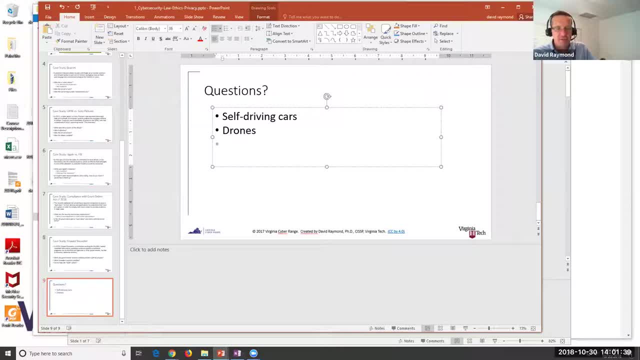 of your drone aircraft that fly over a certain uh ceiling, registered with the faa. so now hobbyists are having to, you know, put markings on their aircraft and share you know and register their aircraft for the faa so that if there's some problem the faa can go find them and you know. 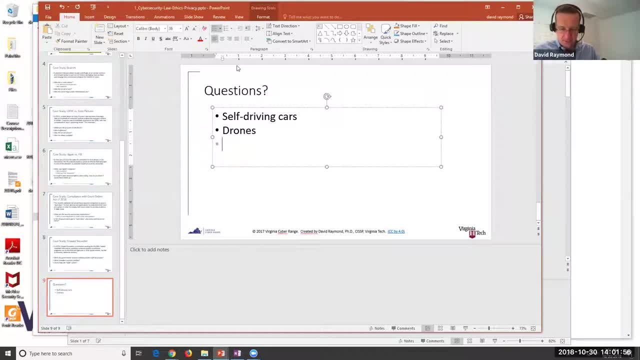 if the drone crashes in a place it shouldn't be, then then they can be- uh, they can be, you know, taken care of by the faa. so that's a big task. um, you know 3d printers- i think is interesting thing to talk about. um, you know obviously very cool technology, but you know what's the future of? 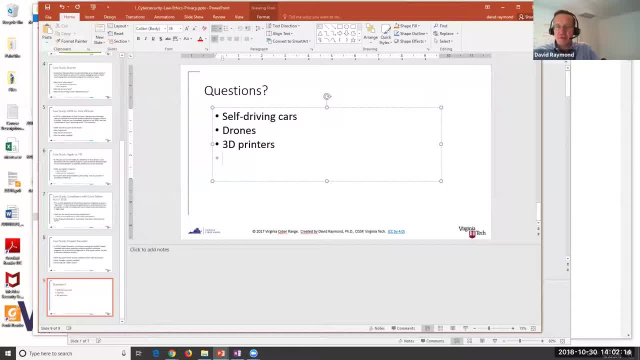 manufacturing if you can. you know, as the 3d printer technology improves and you can basically make whatever you need at home. i mean, there are even 3d printers now that will print in different kinds of metal. so, um, you know, now maybe you don't have to go buy car parts anymore. 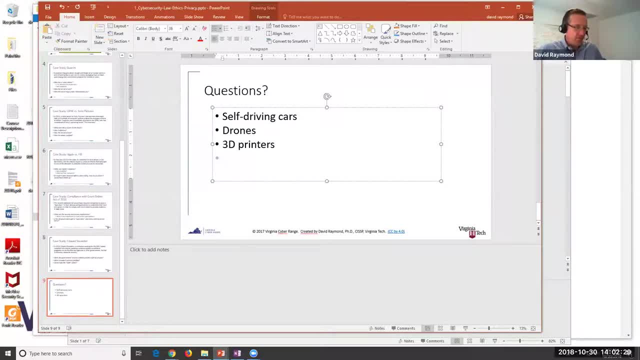 you just download the design and and print it yourself. in fact there are scanners who will scan things in 3d and then you can take that scan and take it over to your 3d printer and print that thing out and um. so that's kind of cool. so 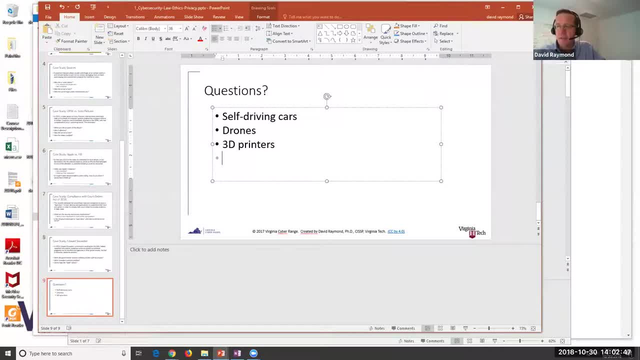 so then you start to get into also, you know, intellectual property discussions. um, you know who owns the design for a physical object, and if somebody scans it in 3d prints, it is that a violation of intellectual property. um, uh, and you know, there's all, there's also. 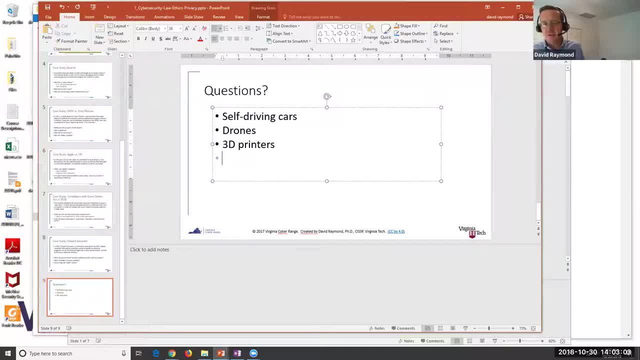 this discussion of: well, people can 3d print firearms. you know that's one you probably hear about a lot. people can 3d print firearms. um, you know, firearm probably isn't going to work very many times if you get it out of your 3d printer. but you know, who knows, the technology may advance. 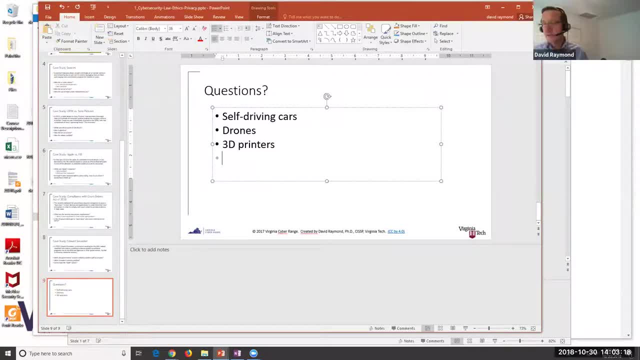 to the point where, um, where that's perfectly practical to print your own guns, and then um, you know. so what are the laws surrounding that? is the? is the 3d model? is that now illegal to possess? um, there's, there certainly has been legislation along those lines. 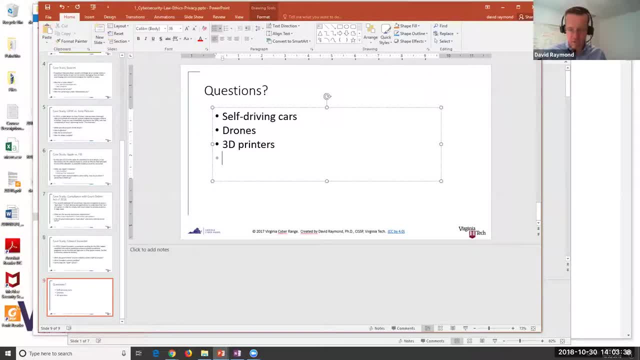 so some interesting discussions there, um, election hacking, um, and there are sort of a couple different flavors of this. right there, there are these influence operations, so what what some people might call information warfare, and this is where you have. this is where you have things that were alleged during the 2016 election. 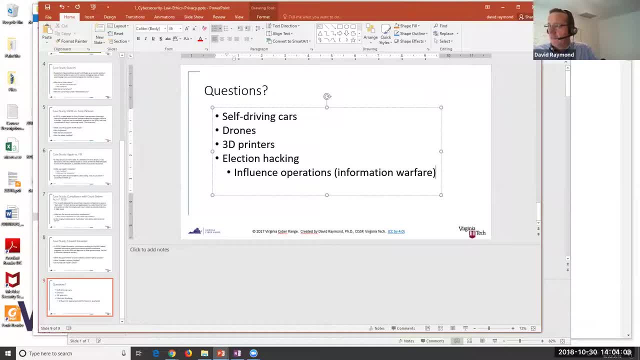 where you had um, these groups who were um groups from foreign countries, who were, uh, using facebook and other online platforms to influence elections, using things like fake news and fake accounts and that kind of stuff. um, you know where do we? you know what are the ethical and legal implications? 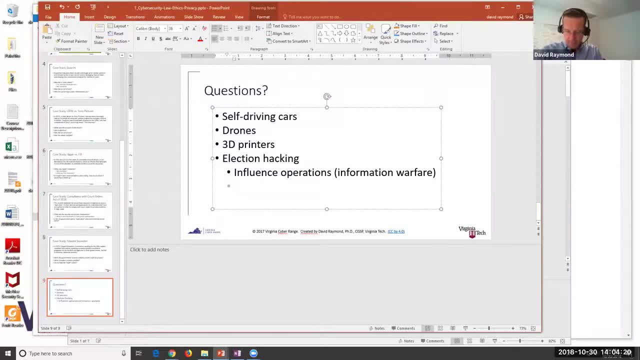 with regard to that. and then you also have, like the um, just like, like the hacking uh of the of the dnc mail servers, mail servers, right, so you had this uh situation where democratic national committee had mail servers that were hacked and you had emails that were taken and shared, and again this 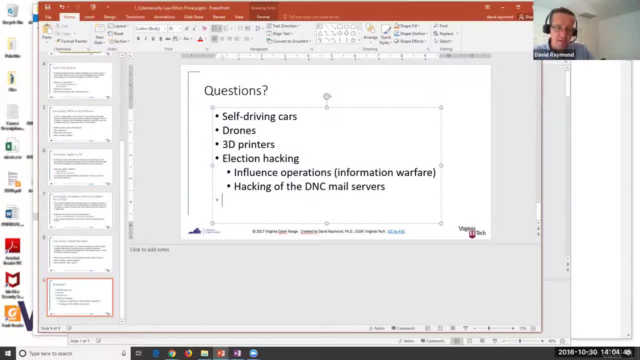 was this all happened to the detriment of the democratic party? there's some things and some of those emails that were that were, um, pretty inflammatory, and so you know what is. is that espionage if that was conducted by a us national? what are the? what you know? what are the laws? 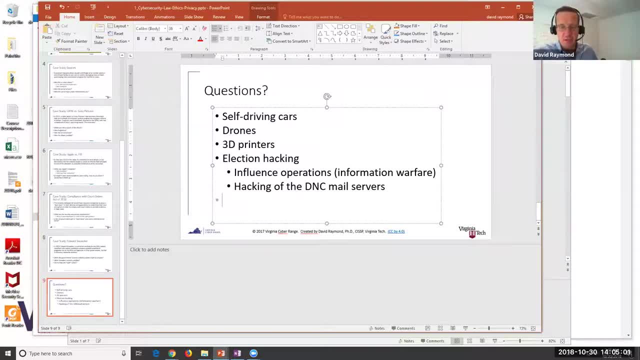 surrounding. if that was, uh, conducted by, um, somebody in another country, what are the laws surrounding that um, what are the ethical implications? do that kind of thing? you know, this is day, this is. this is purely information. it should be shared. right should be. information should be free. we shouldn't be hiding. 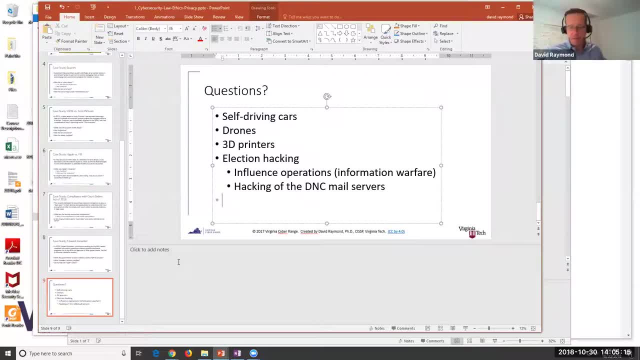 our emails, um, you know. so what are the ethics of it? is that act justified to show that people are corrupt or um you know, or um untruthful or or whatever? um so anyway, just a few ideas. i think there are lots of interesting things that you could pull out and do um these kinds of case studies. i think you could do.